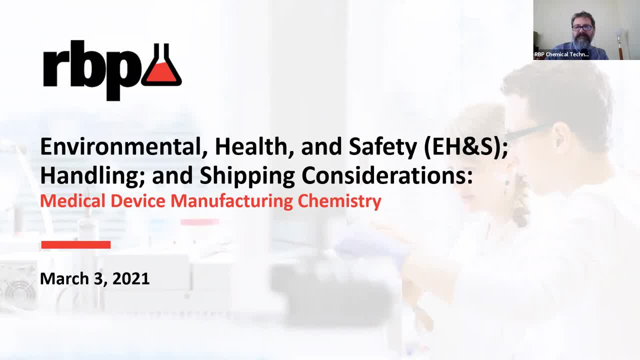 We're going to start here in three minutes. Thank you, All right, We're just going to give it about one more minute and then we're going to start. Thank you for your patience. We're going to start here in three minutes. 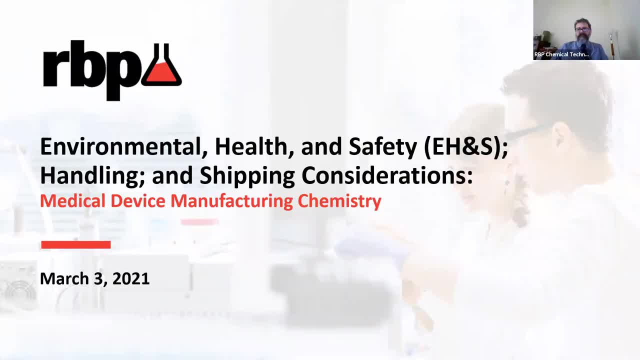 All right, Welcome everyone. Welcome to today's webinar from RVP Chemical Technology, Environmental Health and Safety, Handling and Shipping Considerations and Introduction to Medical Device Technology. My name is Eric and I'll be your moderator today, So a few things about today's webinar. First of all, we are recording this. 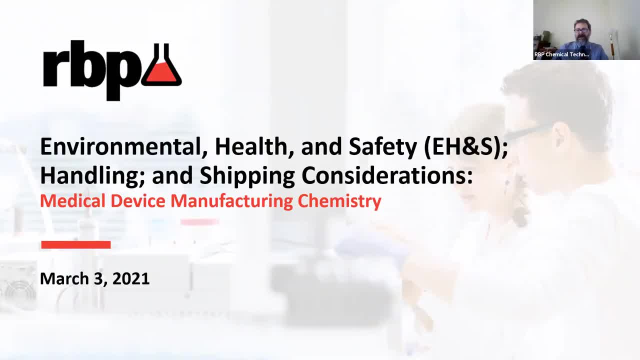 and we will send you a link to the recording to share. Second, this webinar is going to be a little bit more of a video, but we're going to be doing a little bit more of a video. We're going to be doing a little bit more of a video, but we're going to be doing a little bit more of a video. 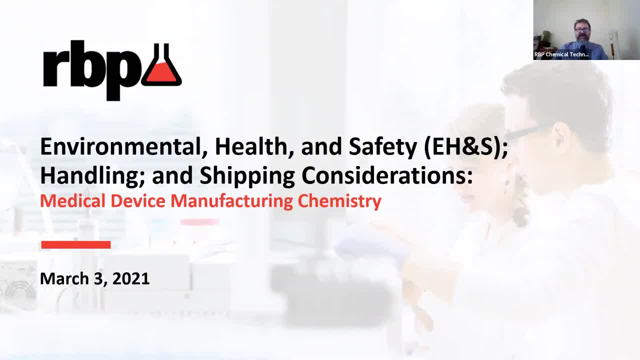 We're going to be doing a little bit more of a video. This webinar will feature a Q&A section and you can ask questions throughout the webinar by clicking Q&A on the webinar controls. If you don't see it, just move your mouse around and the controls should pop up. 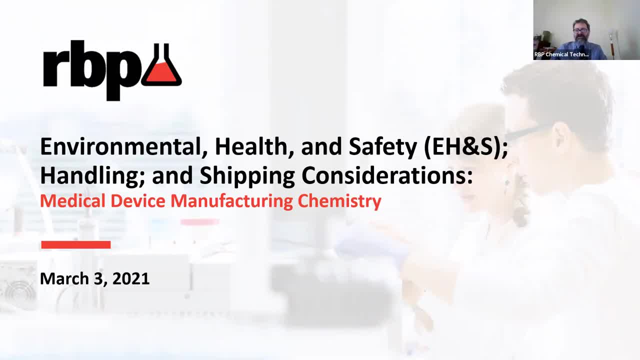 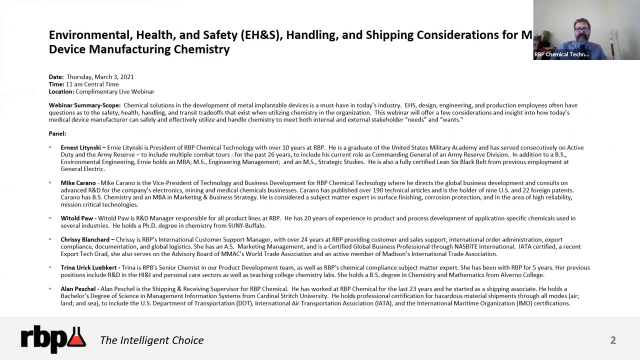 We will also be monitoring the chat, if that is an option on your screen. We'll be answering any questions you may have at the end of the webinar and we'll try to get to as many as we possibly can. All right, so the scope of today's webinar will be chemical solutions in the development of metal implantable devices. 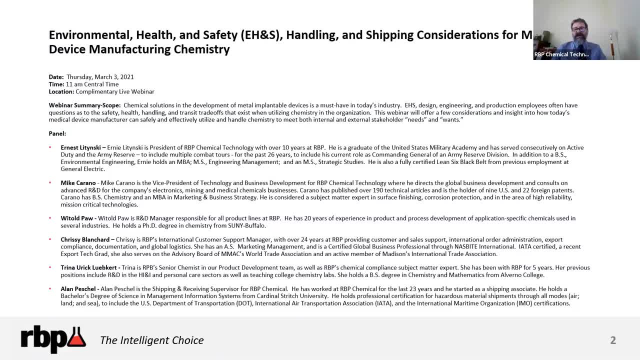 EHS design, engineering and production employees often have questions as to the safety, health, handling and transit trade-offs that exist when utilizing chemistry in the organization. This webinar will offer a few considerations and insight into how today's medical device manufacturer 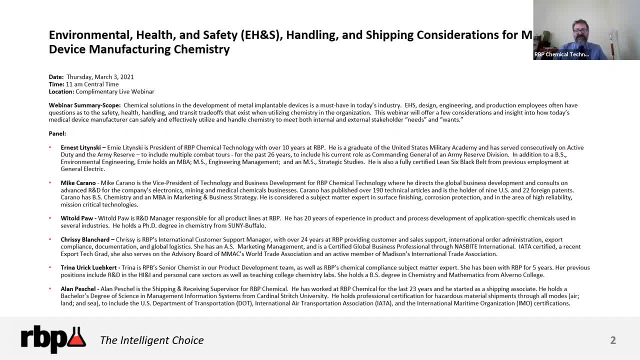 can safely and effectively use chemical solutions in the development of metal implantable devices, EHS design, engineering and production. employees often have questions as to the safety, health, handling and transit trade-offs that exist when utilizing chemistry in the organization. 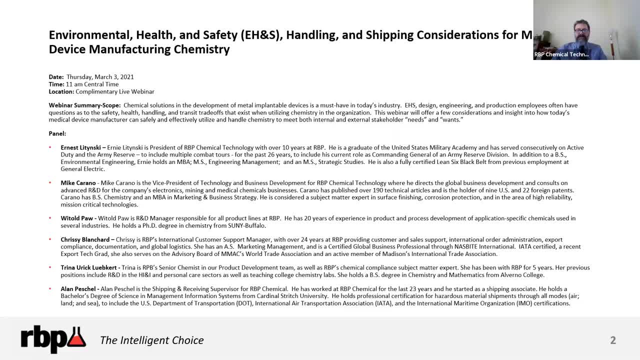 All right, oops, sorry about that skipping ahead here. Now I would like to introduce you to today's panelists. Ernie Lutensky is the president of RBP Chemical Technology. Mike Carano is vice president of technology and business development. 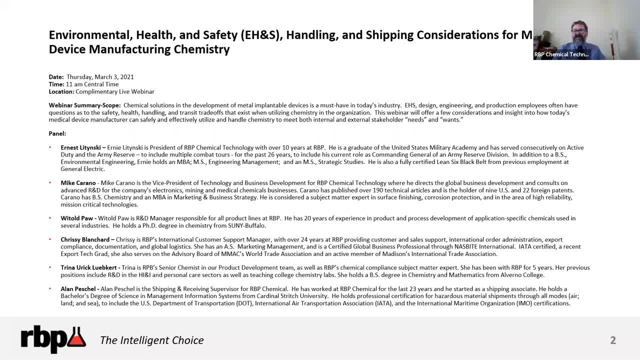 Vito Paul is R&D manager responsible for all product lines at RBP. Chrissy Blanchard is RBP's international customer support manager. Trina Jurek-Lubkert is RBP's senior chemist in our production and development. 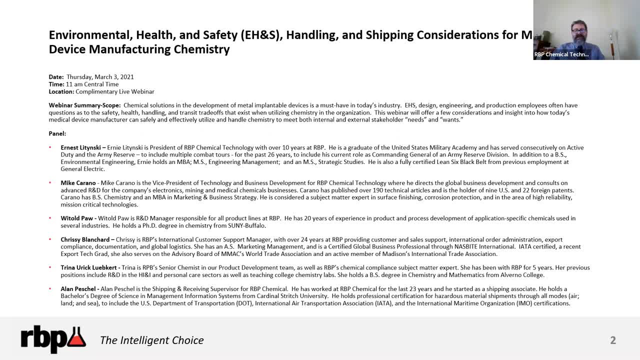 or product development, And Alan Peschel is our shipping and receiving supervisor. So we're going to start today by an introduction to our first speaker, Ernie Lutensky. Ernie has been with RBP Chemical Technology for 10 years and is president of RBP. 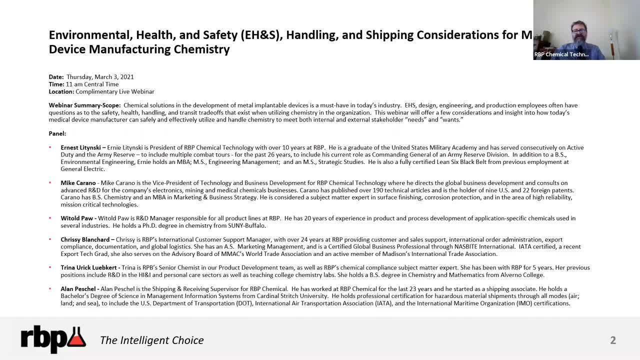 He is a graduate of the United States Military Academy and has served consecutively on active duty and the Army Reserve for the past 26 years. In addition to a bachelor's degree in environmental engineering, Ernie holds an MBA in engineering management and another master's degree in strategic studies. 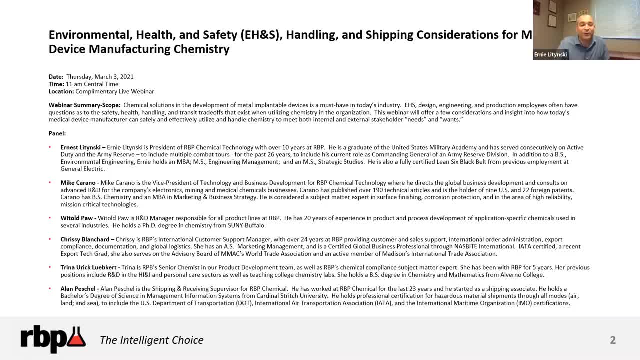 Ernie, take it away, Eric. thank you. Thanks for the warm introduction. Hey, to all our partners and folks on this webinar, I would like to say thank you for taking the time here today. We pride ourselves and I think you'll see this a little here today at RBP. 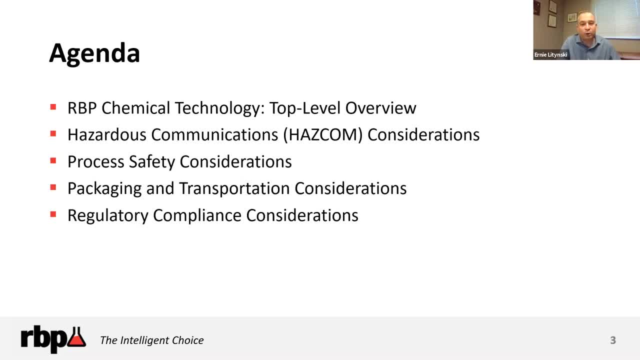 to winning your business and partnering with you long-term for what we do day-to-day, And I think we'll offer a little glimpse into one of the things that we could hopefully help you with here going forth, and that's environmental health and safety and everything all about chemistry considerations. 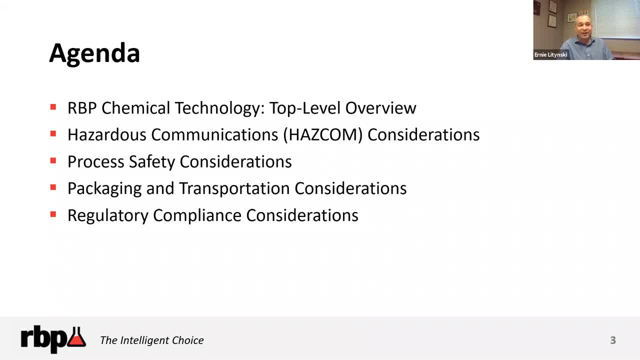 Although chemistry may seem a little dangerous, I will tell you. I think once we do this webinar, you'll see that chemistry exists all around you, to include drinking a Coca-Cola or a Pepsi, which could require a safety data sheet as well, you know. 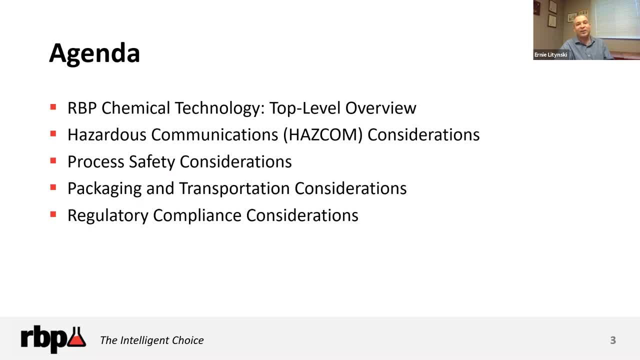 based on the chemicals in there, and in this case phosphoric and citric acid, among other things. So I would like to walk you briefly through the agenda. all right, We'll just give a. I'll give a 30-second elevator speech on RBP chemical technology. 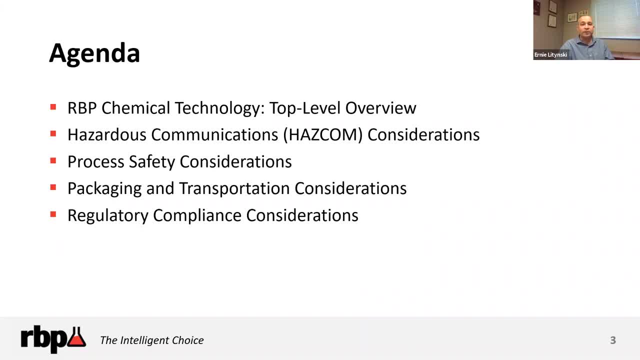 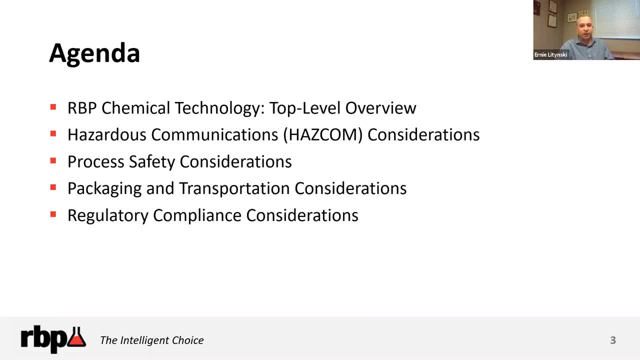 for all our employees for hazardous communications, because I find that to be one of the most important things to know and is a right to know of all employees and all folks that deal with chemistry within our up and down, our supply chain. At that point we'll hand it over to Dr Vitold Poth to talk about some. 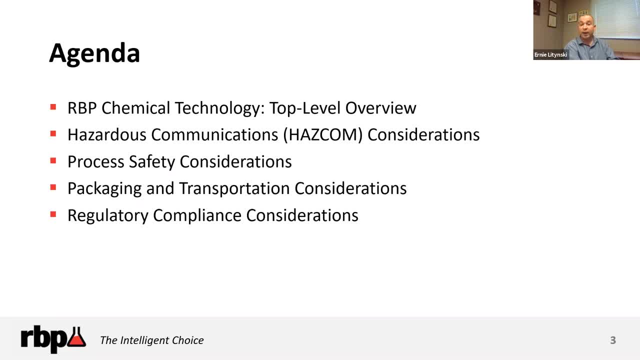 of the process, safety considerations when handling and utilizing chemistry. and then we'll go into, Chrissy Blanchard, on packaging and transportation considerations, which we often take for granted, you know, on how to ship chemistry via different modes and mediums of transportation. and finally, we'll wrap up with a couple regulatory compliance. 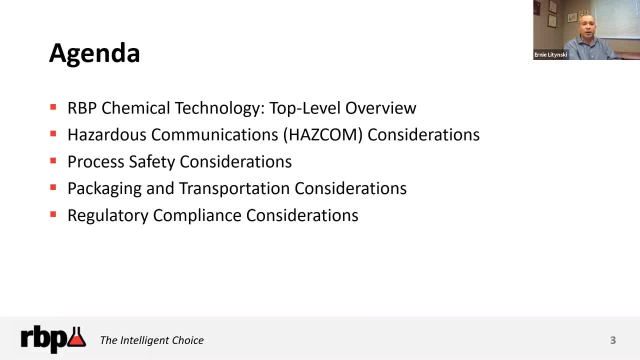 considerations that Trina will provide to us. be it known that in all these considerations we may or may not have the right answers, but we are willing and dedicated to assist, both on this webinar and post webinar, to help you on a daily basis to make sure that you know what. 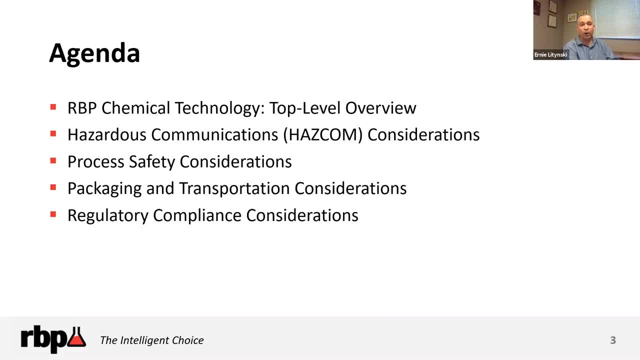 you're doing with our chemistry, both from a process perspective and performance. but the focus here today will be, you know, on health and safety of your employees as we utilize chemistry, whether it's RVP's chemistry or assistance you may need with a another chemistry you already use, and again, that's what we're dedicated to: partner with. 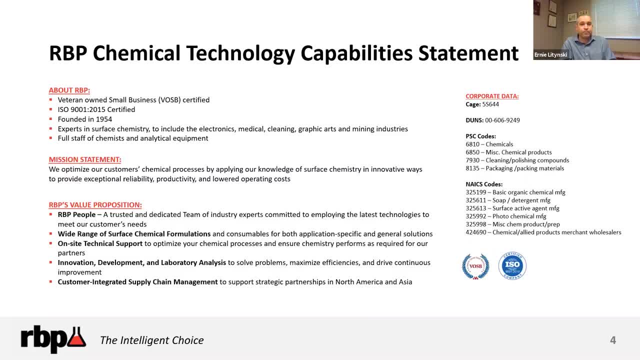 Eric, if you go to the next slide real quick. so just a little about RVP chemical technology in this capability statement. COVID, world wars, you know, whatever it may be, we are and have been around since 1954.. You see the third bullet there we take a little bit of pride with being a veteran-owned small. 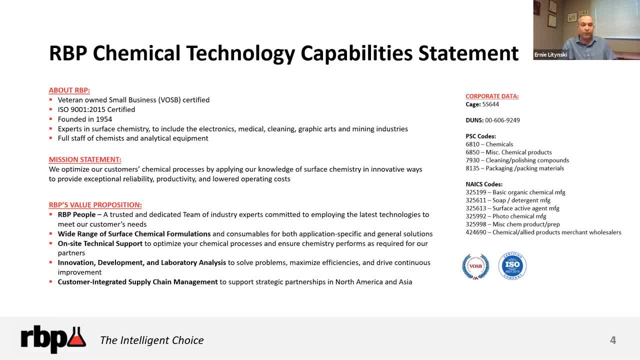 business. so we're in essence a minority business with veteran status, and by veteran, our our owner and CEO, Mark Canneberg, is. he's also a West Point United States Military Academy graduate and fought in a couple conflicts in Vietnam. so we're proud to have that status and support, you know, service members and others with with small business. 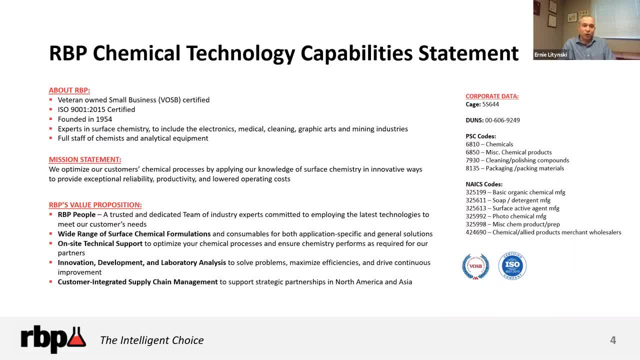 classifications, you'll see that we're ISO 9001 2015 certified, all right, although we have the status for about, you know, two decades. we're really on the path of doing a lot of work in the field of lot of other things, with gmp iso 14 000 uh in in a couple other certifications, although we may or 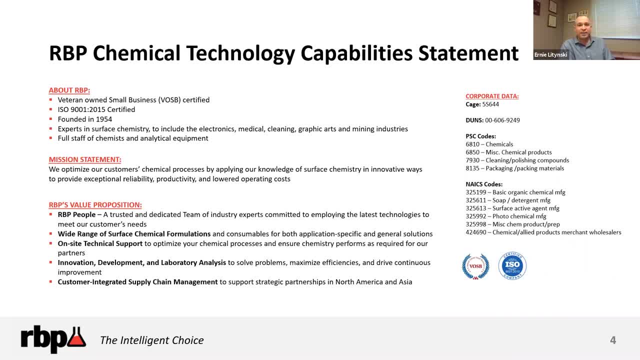 may not qualify, in some instances we do use those best practices. so that's something we take to heart for all the chemistry we make and working with our partners. all right, third bullet there, or correction, fourth bullet, although we're in medical device manufacturing and printed circuit board and 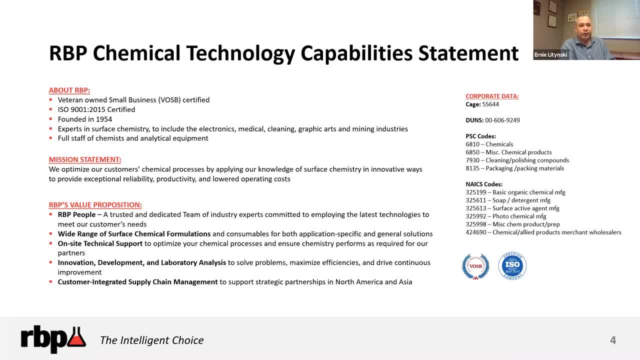 semiconductors and graphic arts and in mining applications. really, at the end of the day, would you know, since i've been here in the team that you see in front of here today- what, what we really take pride in is our core competency, and that's being experts in surface chemistry. so it's really 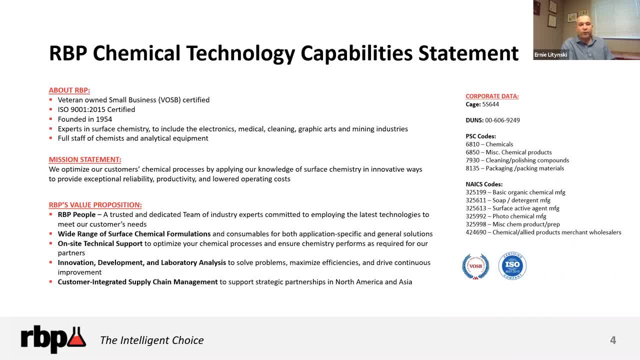 understanding that that function of you know cause and effect of chemistry with whatever medium. you may think that's not a big thing in a printing press room, all right, all the way to medical chemistry. but i'm going to use printing test room press room as an example. you're touching many 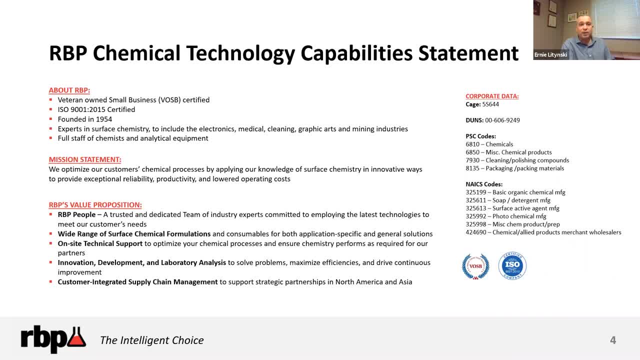 different surfaces. you're touching many different surfaces. you're touching many different surfaces there. you're touching everything from organic, with paper to aluminum plates, to polycarbons and hydrocarbon substrates, plastics, all the way to using other chemistries in the case of ink. so that's what we take our pride on in doing and we and we want to do it safely with. 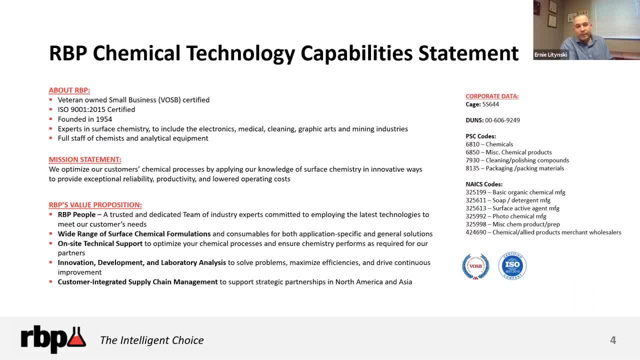 handling of chemistry. all right. the final bullet there about rbp is is: we're not a transactional organization. some of the folks you see here on this call today will help you out with with somebody who's environmental health safety. you know shipping and handling considerations, but the 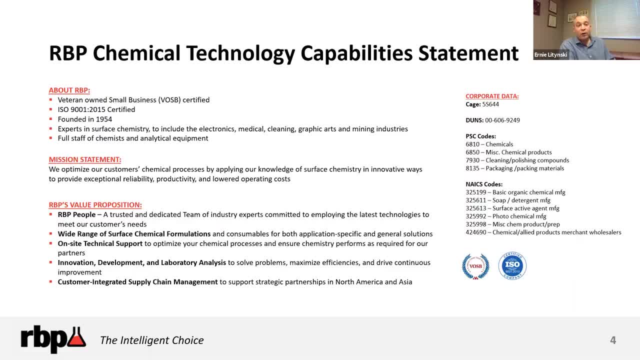 likes of. you know, trina and vetoed, present here today, those chemists. you know, full staff of chemists. in addition to them, we have other chemists here. they're the ones that help us figure out. you know, what we can do to better your organization with, which is really our. 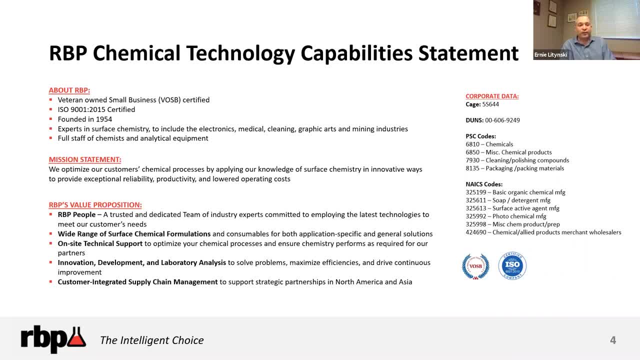 mission statement there. so we're. we are, as a privately held company, committed to optimizing your processes by applying our knowledge as it states there, and at the end of the day, it's you know, not having the ability to fail for a medical device, so we need that reliability. 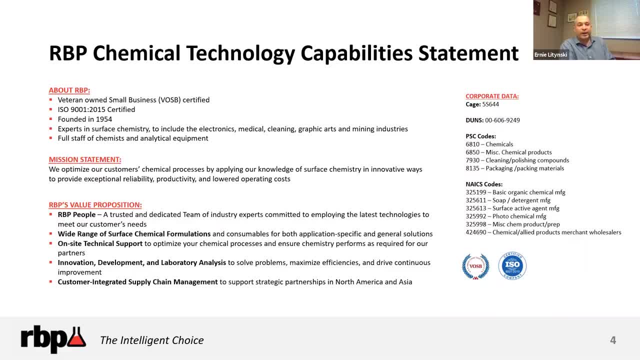 we acknowledge your stakeholders need productivity and we acknowledge that you know we want lower operating costs to remove the non-value-added processes you know in products out of your product line. so again, that commitment from the mission statement flows right into our value proposition and, you'll see it, we have a dedicated group of people here and that's why we're taking 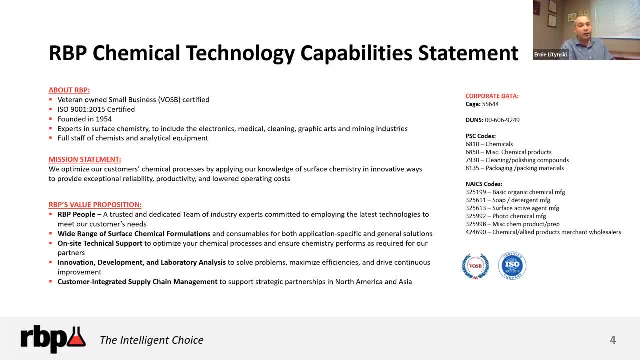 the time and we appreciate your time. i'm doing this webinar here today. all right, we could figure out a wide range of surface chemistry formulations, whether it's an off-the-shelf product or something for your specific needs from a performance perspective or from an environmental, health and safety perspective. 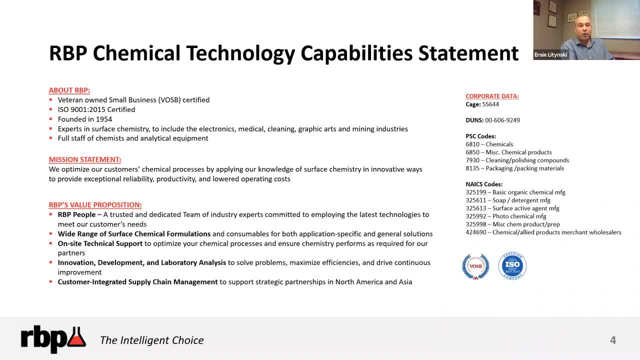 as well and and dedicated with that formulation goes the on-site tech support. you've got a couple folks on this call today and mike carano and and trina and vetoed that will come on site and help you optimize and do what we need to do, but more often than not we will help you innovate, develop. 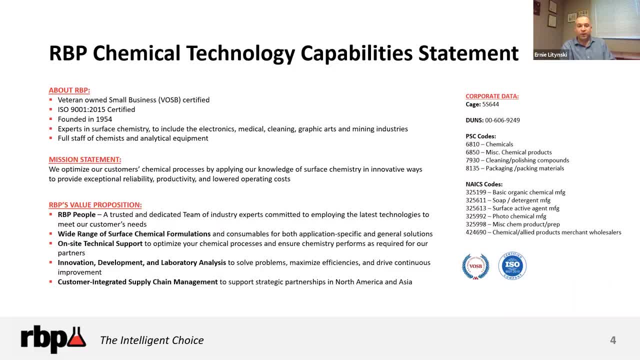 your solutions and navigate through that toolkit as soon as possible. so thanks for that and i'm happy to have you here today and we're going to wrap up our webinar today. thank you so much for coming in and thank you thanks for having me. i'll see you next time, on the next show. 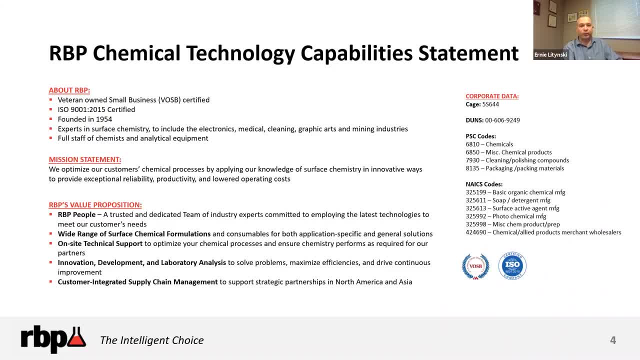 you're looking at that. uh, that's your, uh, that's your first bullet point, right, and you're looking at that. so i'm glad you're with us today and i'd like to thank everyone for joining them. i'm going to see if you could bring up your starting point in a second and give. 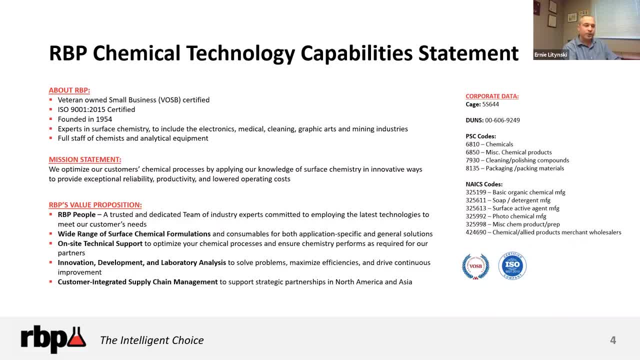 you a little bit of context. so if you could take your time and i'll see you in the next product session- see Blanchards and folks internally here. we will figure out what we need to do strategically for you to make sure that supply chain is both safe and meet your internal requirements. So enough. 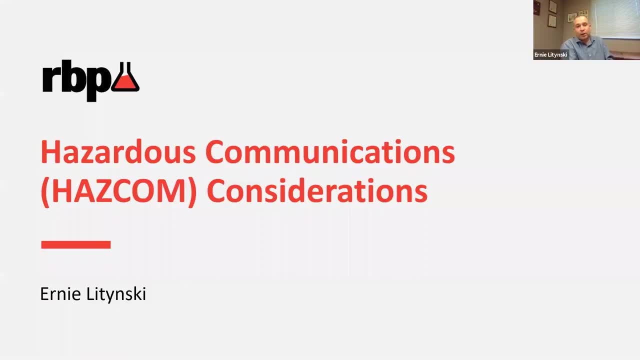 about RBP. you know we want to get into me to this and help you out a little, And I wanted to start with probably what I see as the most important piece with chemistry in any industry, and that is hazardous communications. So we'll talk about a few considerations here Again. 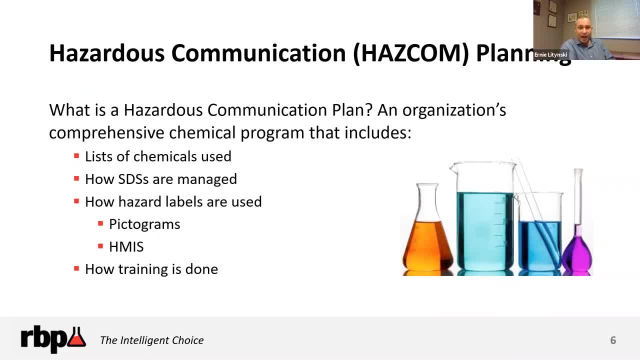 this would be more of a blanket top level. look on planning with HAZCOM. But if you have any questions, hey, you're talking to the guy that we find important enough, you know, with Trina and Al Petros and others here, you know, to write our plan because we think so highly of being safe here. 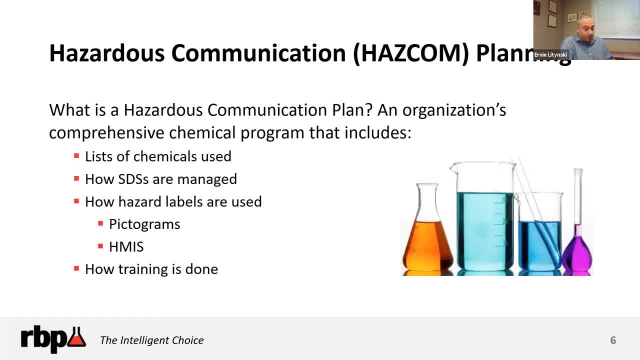 So with hazardous communications, I will tell you, and we could give you more on this, but there's something called, you know, OSHA recordable incidents. you know, which we have to report to OSHA for incidents that may occur in our plant. 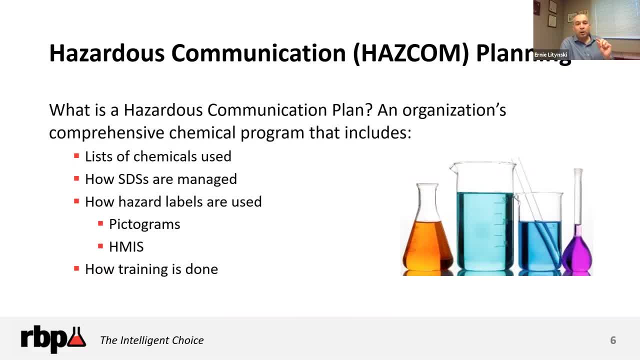 I'm proud to say we have not had a chemical OSHA recordable incident for 19 and a half years. right now. We've had OSHA incidents but things happen, People, you know you have slips and trips and falls. The actual last OSHA incident we had- and this goes to the pride that these people have- 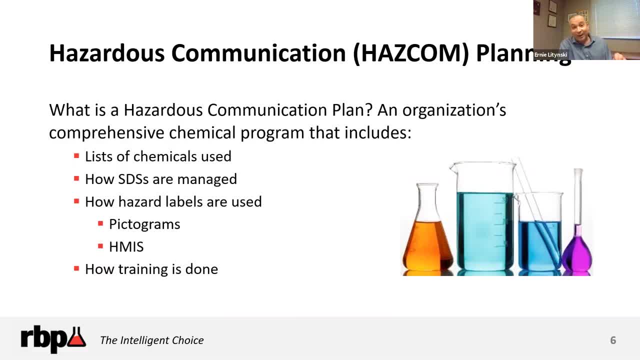 on this call. here was actually a slip in the parking lot on snow. So sort of stinks to live in the north. but that goes back to where we've had for an OSHA- you know- recordable incident. that goes back now four and a half years. So we take pride in this, So you may ask. 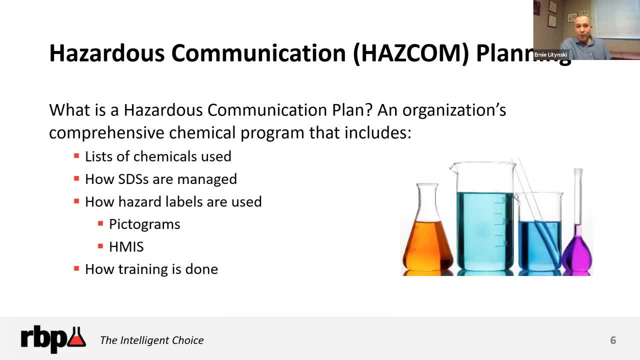 yourself what a hazardous communication plan is. all right, We've got one here, but I wanted to share some best practices here on what I propose you have in it. all right, at a minimum, And you'll see what it really is here. It's an organization's comprehensive chemical program that includes: 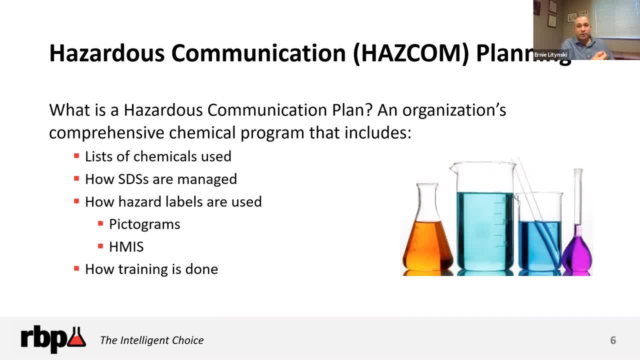 a list of all chemicals that are used in-house, all right, And it goes everything from you know, say, RBP chemistry to you know the use of chemicals that are used in the house, And it goes everything from you know the use of chemicals that are used in the house to potentially 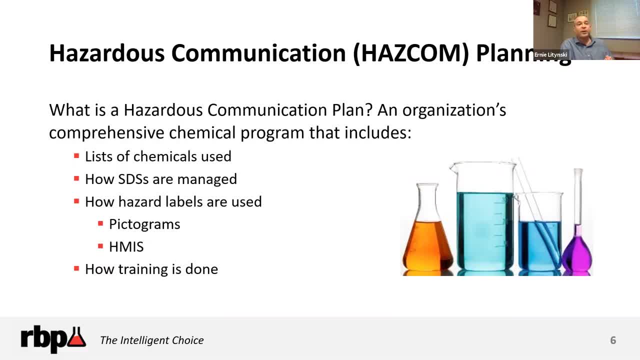 compressed gases to potentially cleaning supplies that you have in-house, And we've got a subject matter expert here that helps me out a lot on this And Trina, she'll come up and correct it. We bring a new chemical in with our cleaning team here. We need to know that there's a right to know. 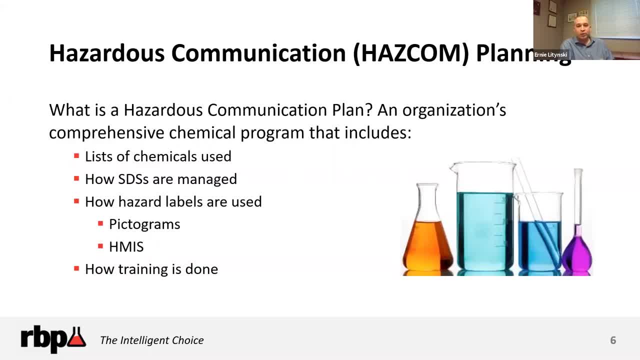 of every employee in your facility, of a list of all chemicals used. all right, And the way you really manage that is through something called a safety data sheet. We'll talk about that a little more in the next slide, But in the past you may have heard the term safety data sheet, And I'm 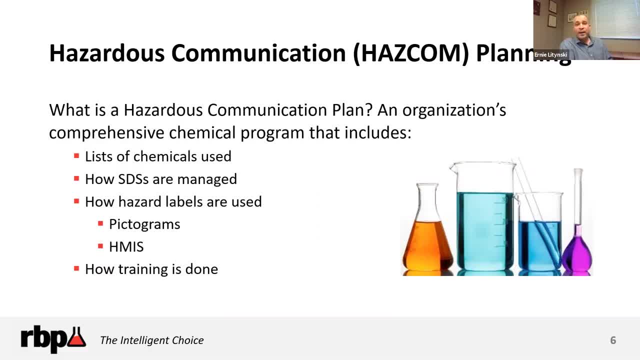 sure you've heard the term material safety data sheet. okay, But now it's a comprehensive document called a safety data sheet, with 16 sections, So we want to know how we manage them. We have the most up-to-date safety data sheets as well, And this is important because, again, all employees have a 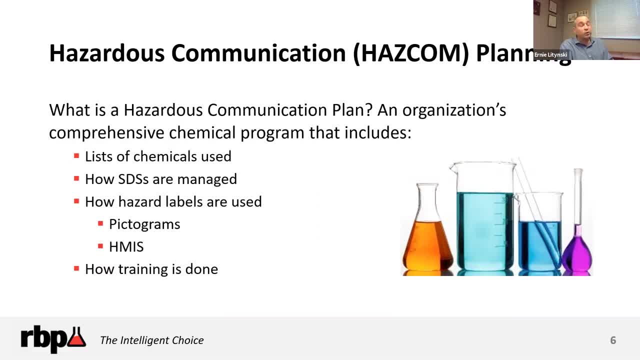 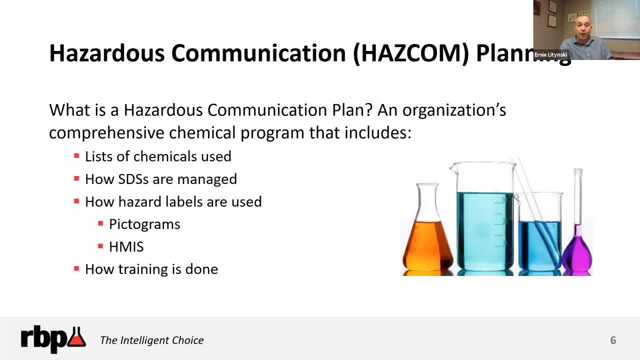 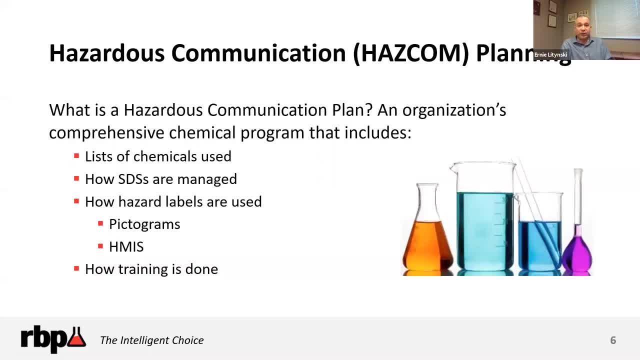 you'll see something called a pictogram, okay, on a bottle, Okay, And you'll see a pictogram tell you what the dangers that exist are and then what level those dangers are. All right, And that goes right into the identification system right there as well with the HMIS. So you'll see that the 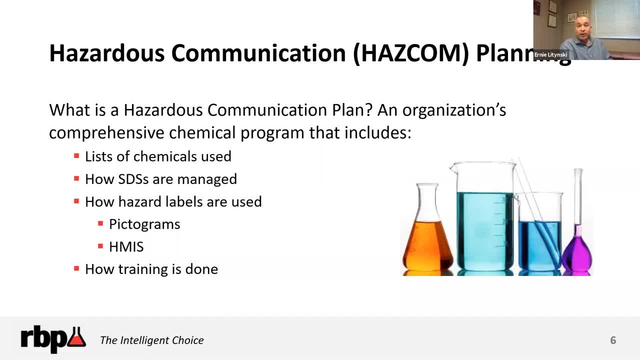 you'll see certain statements. What I will tell you is when you start building this hazardous communication plan. you will see all this on our safety data sheets, as well as whoever else's chemistry you may be using, And again from the beginning of your supply chain or what you have. 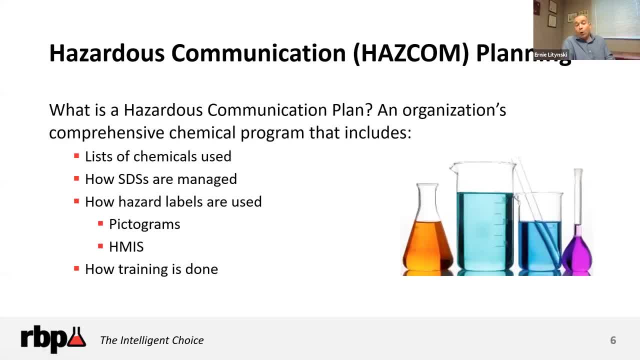 in your facility all the way to the end, right? We're more than willing to help you out with this and understand it. all right, I will say once again, Trina, I'm throwing it to you, but we have a subject matter expert that's dealt with this for many, many years in her career and we are 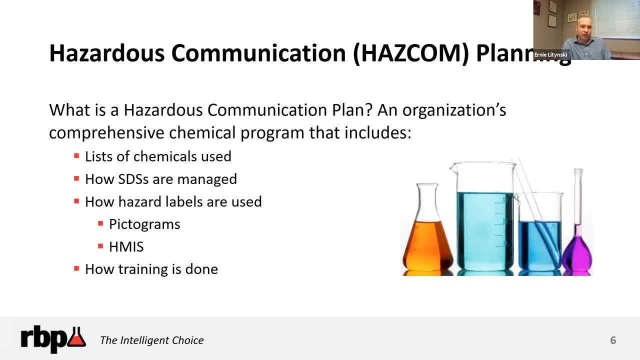 dedicated to assisting from Trina and Al Paschal and others here. all right, So that's the three top bullets, and the last one, which I see as the most important, is how training will be conducted on your hazardous communication plan For our employees. here we've got what may seem, you know. 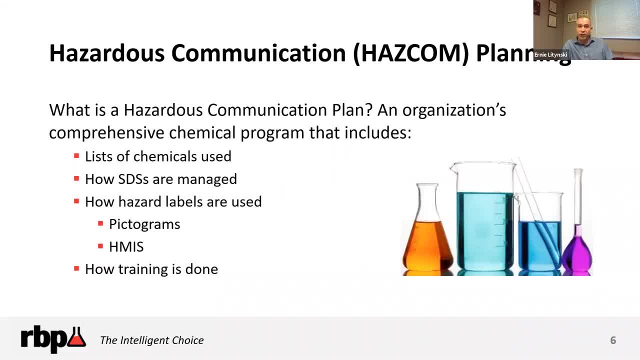 death by PowerPoint: 27 slides in annual communication, but it's more than that. This is where we seek feedback from employees. when we do that training piece, you know, with best practices and how to up our game a bit more in everything we do. So that feedback mechanism during training is very important. I'm very 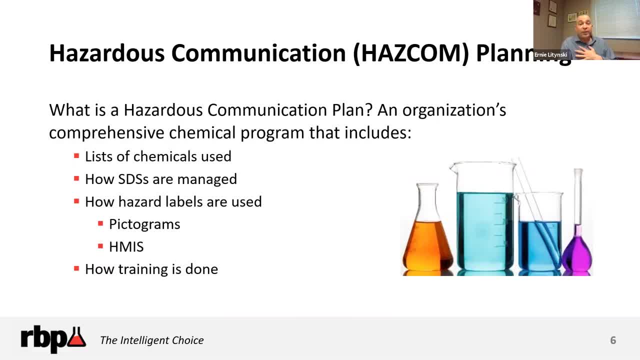 willing to, you know, redact a few things in our plan. but again, this hazardous communication plan with these four main bullet points really is the structure of what every organization should have, and I am personally committed as president here and what I consider a subject matter expert on. 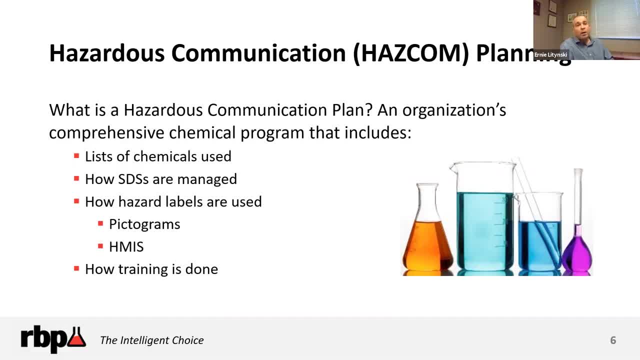 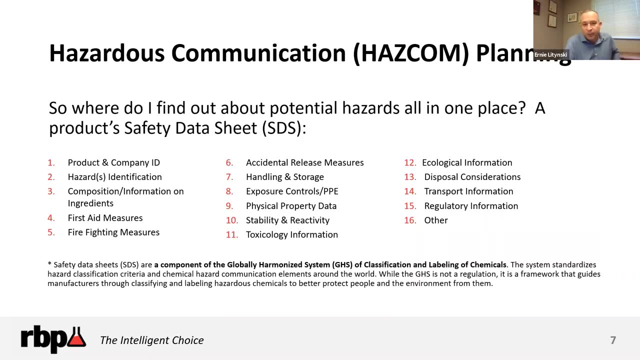 HAZCOM To provide that to any participants on this webinar or please pass it forward to anybody else in your organization or that supply chain. there you know post-webinar here. So with that said, I'm going to touch one more thing on HAZCOM, which is really the meat of how your HAZCOM plan. 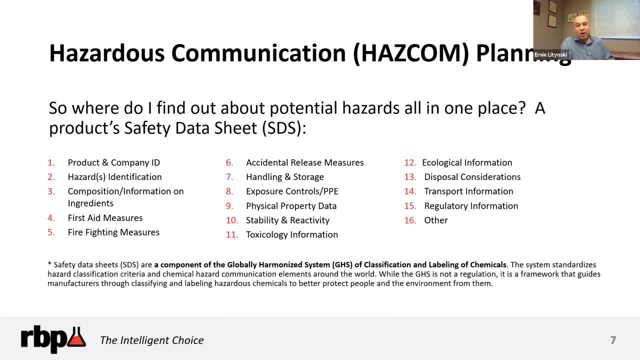 starts and how you start creating it, and that is something called, as we talked about this safety data sheet- or, you know, pre-2012, a material safety data sheet. On any safety data sheet, you'll see there's 16 separate areas of it. This will tell you everything you need to know. 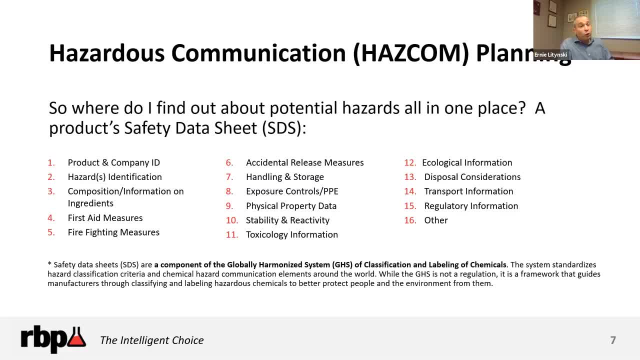 about a chemical and again this goes back to, you know, having a safety data sheet for bug killer around your house or a fertilizer. all right, Those, you could request those and you could get those. and for our chemistries, we have these and we have a good deal of detail on these. 16. 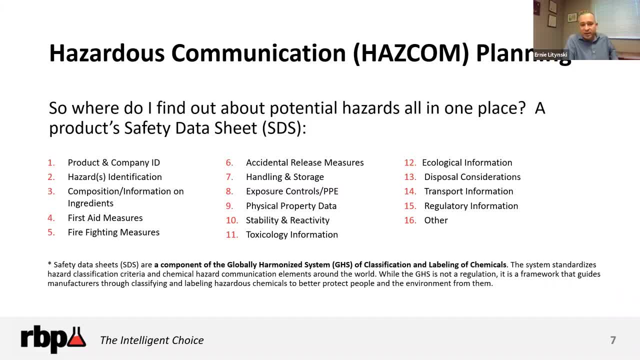 areas. all right, I'm going to take you down before we talk about some of this in these 16 areas. to to that little italicized thing: what a safety data sheet is? It's really, it's just one small part of of GHS, this globally harmonized system of classification and labeling of chemicals. 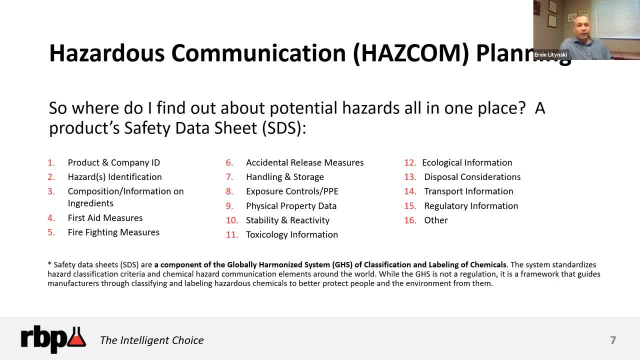 all right. What you'll see is that many countries may have different nuances to a safety data sheet, but most of the most of the world has adopted what is these 16 areas here in a safety data sheet with GHS. So they've taken the framework you know that's put out out there by the 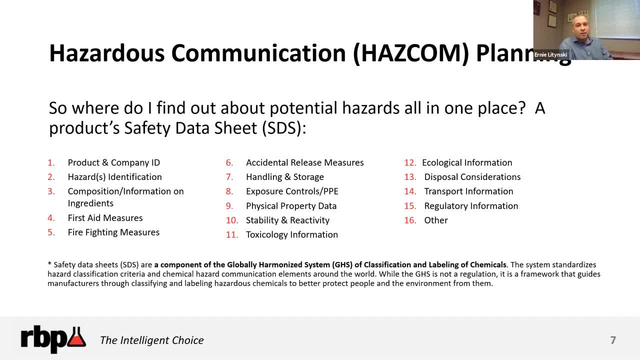 global body and you'll see, in many cases it's, it's, it's almost the same and identical with these 16 areas, all right. And again, it provides that framework. It's not a regulation, all right, But there are regulatory portions of it, but it guides the manufacturer and then all users to keep. 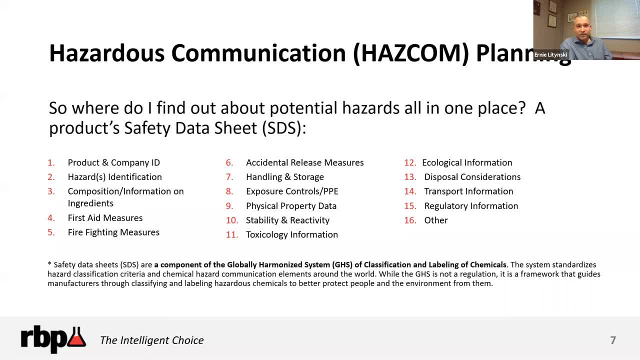 people, flora and fauna and then the environment overall- safe in what we do every day. We will touch on a few things here in in in the safety data sheet today, but I will try to take you to, you know, a couple points here. 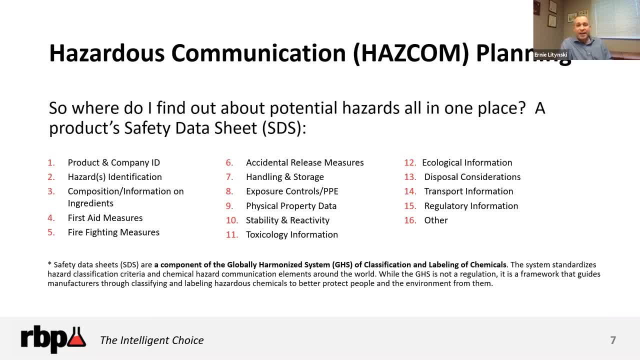 I'll, I'll, I'll talk about, you know, number six a little bit on the next slide with accidental release measures, and I just want to use that as an example to everybody on this webinar and your organization's post-webinar as to you know how we could help out a little if you do have that spill. 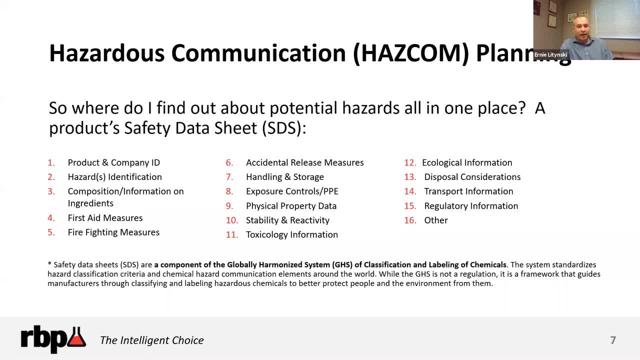 or an accidental release. We'll talk about that a little in the upcoming slide. Chrissy and I will talk about the handling and storage piece. You'll hear continuously about PPE, and PPE stands for personal protective equipment. So that's everything from you know wearing maybe. 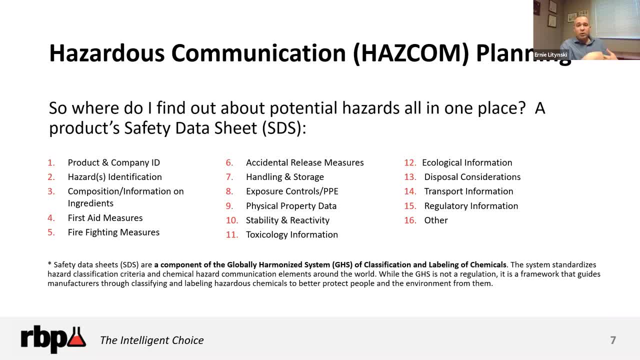 basic gloves when you're at home using a fertilizer. all to a to potentially. you know devices and controls and engineering mechanisms put in your facility you know, as well as personal protective equipment that you may want to have on your body when dealing with specific. 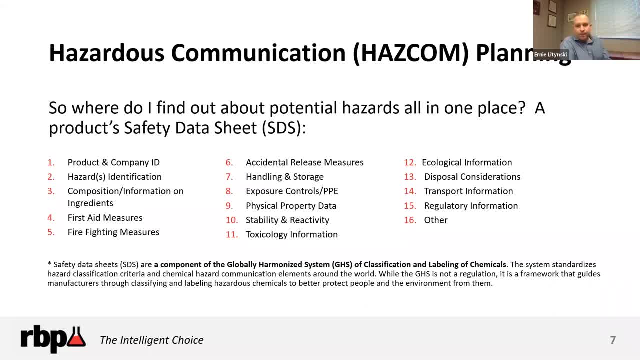 things, And then we'll give you some options on on how to mitigate some of these risks. All right, We'll also talk briefly here today on on number 14, transportation information, which will be handled by Alan and Chrissy. 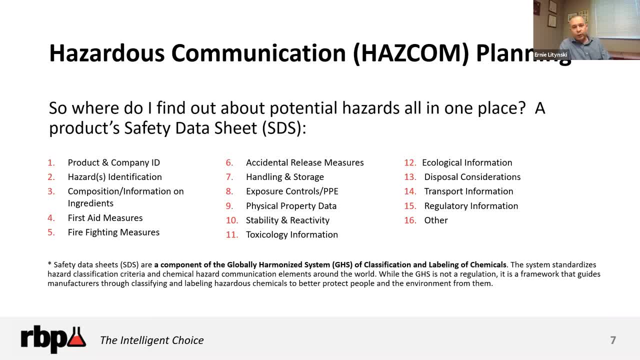 and then number 15 with regulatory information handled by Trina, The reason we're touching on these. I mean we could do this webinar for hours. We find these oftentimes are really the most important pieces. when you start talking and understanding, you know how to work and what. 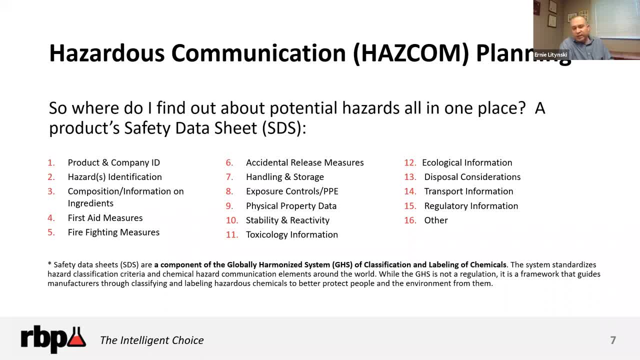 considerations you need with chemistry. So we'll hit, like I said, number six, a little number seven, we'll touch on eight and then we'll hit, you know, 14 and 15 in more depth here with with my fellow speakers here today. So, with that said, I was going to take you to the next slide. 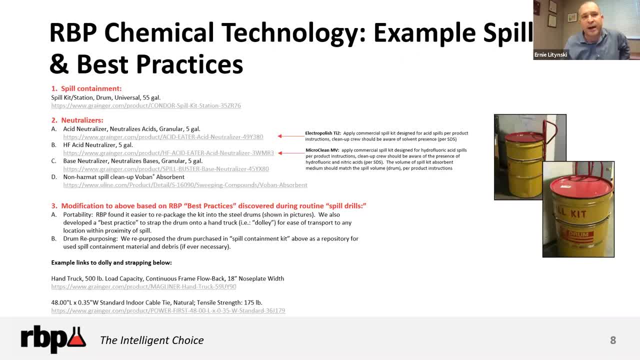 and show you some things that you know you develop over time as a best practice. and look, not one specific person developed this, but just wanted to use an example that you know. maybe we provide some of our partners. All right, So what we did internally here is we actually? 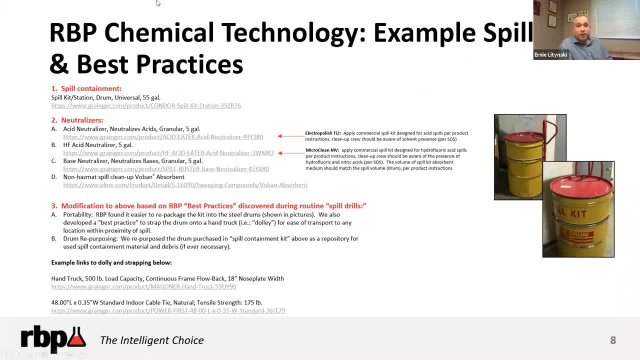 developed a spill kit. So you have spill kits throughout the the facilities, both in a lab environment, you know, with VTOL and team, all the way down to manufacturing and then all the way through the end of our line and our shipping and receiving. 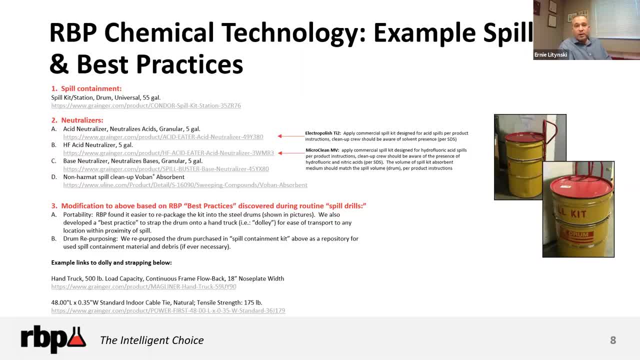 doc, where Alan Peschel, who's on this call here today as well, has responsibility for inbound and then outbound- you know chemistry- for our facility. So I'm just going to use this little anecdotal example here of what we do and maybe some of the value we provide, and you know, 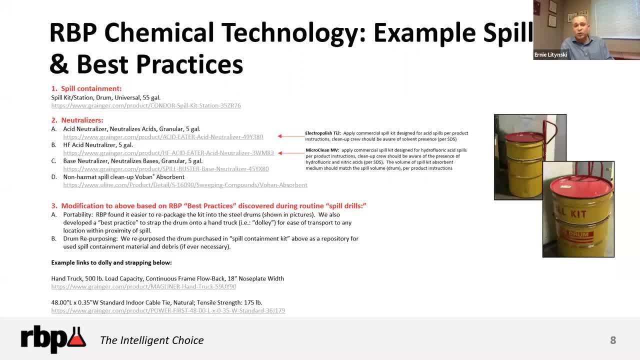 we could work through for your specific needs. But a consideration is: once you know the chemicals, you know you're, you're going to need some kind of kits. Like I said, we use a drum, the lab uses smaller. you know things, but what is part of that kit? You know, and this is 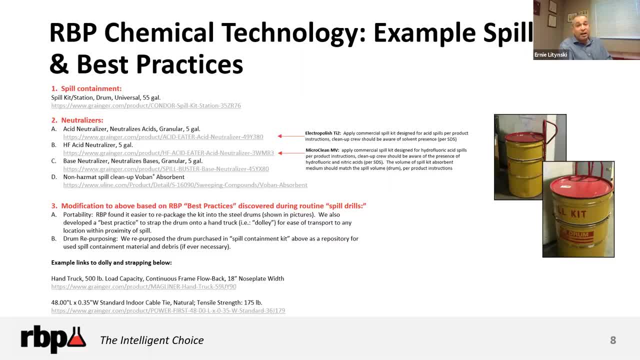 this is some things you may want to think about in your organization. based on the safety data sheet and knowing the hazards, you may need a acid neutralizer right Or a base neutralizer, And you'll see in number two a here or correction to a and B. just give a couple of different. 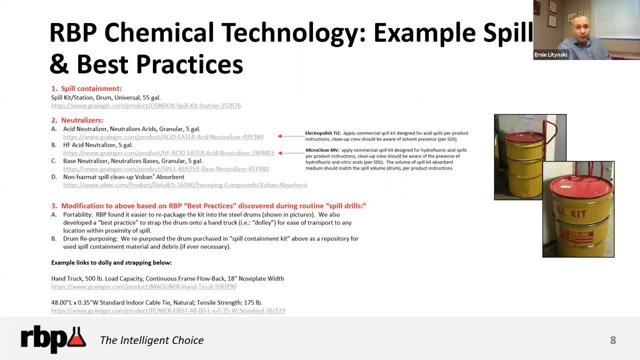 examples. So we have a couple of products, electropolished GI too, And for that one buy a acid neutralizer and we have a link here. You know we're not endorsing anybody. You go to something simple as Granger and buy that specific neutralizer and, and you know, have it in your 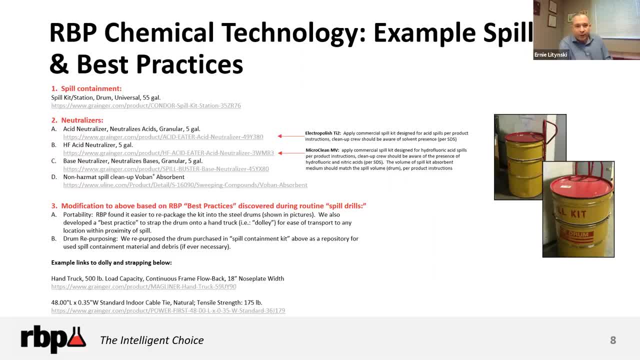 location. And then the same goes for you know the, the next one here, you know, based on a HF. you know if you're using hydrofluoric acid in it, so got a base neutralizer, and then we've really got some absorbent best practices as well. So you start talking neutralizers. 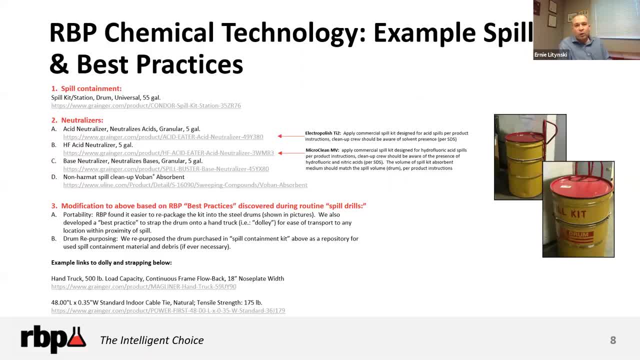 which is a key portion of a kit. Let us help you with that you know, or give you some you know, some advice and ground you if you're going down this direction. All right, So the the big things that you see, oftentimes too, for your organization is bullet three. All right, We may have something. 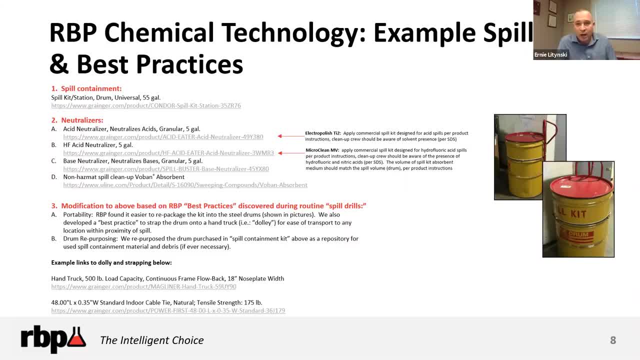 here internally, but what we want to provide you is that value added. when you're talking to a Mike or a fetal or, you know, Trina, when you're looking at doing something in your process line is: Hey, how do I make this thing tailored from our organization, our organization, right? So in 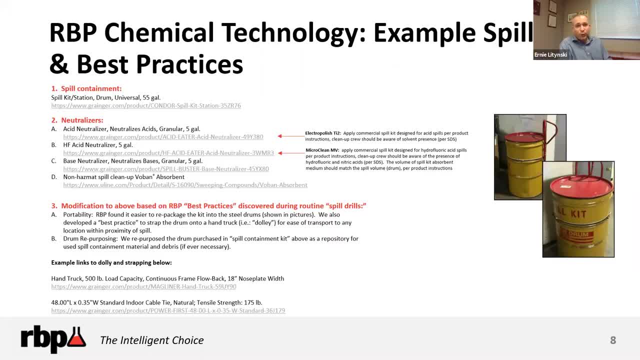 your case, your organization. So for us, you know, portability, there's simple things that can happen. You got a drum, You know we- just Al Paso came up with it with his shipping guys. Hey, let's put it on a. 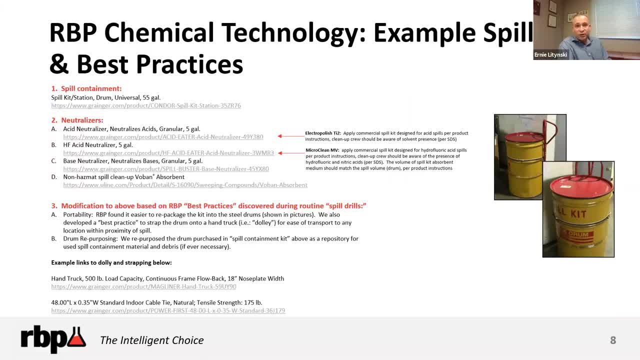 I'm going to lose the term here- a dolly right Or a hand truck for easy transport Right. You may want to have modularity. So everything in that drum, from a spit, you know from, from dyking to sorbents to, you know, neutralizers, you know it's self-contained. 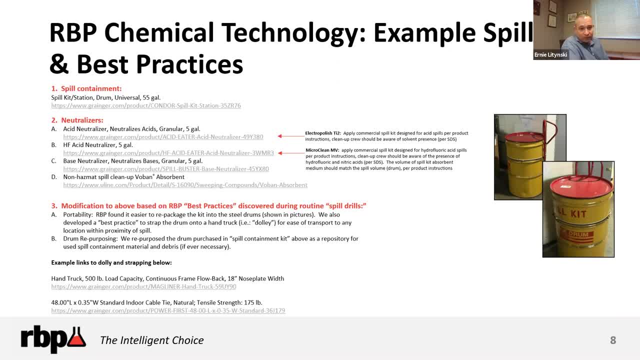 All right. So just an example: right, And then drum repurposing, right. So we we also have an area where you know you have sorbent materials in in debris left over and we do spill Spill exercises here. regulatory, We have a regularly. we have two different alarms. 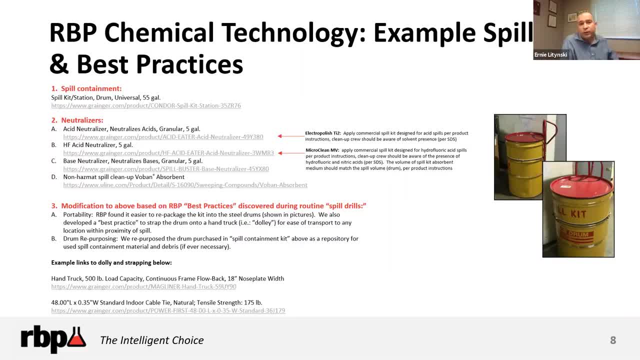 one for fire, one for chemistry spill. You got to start thinking through some of these things and you know, practice makes perfect on the path to continuous improvement. So, again, this is just, you know, some of the things we learn internally, some of the best practices that we're. we're very 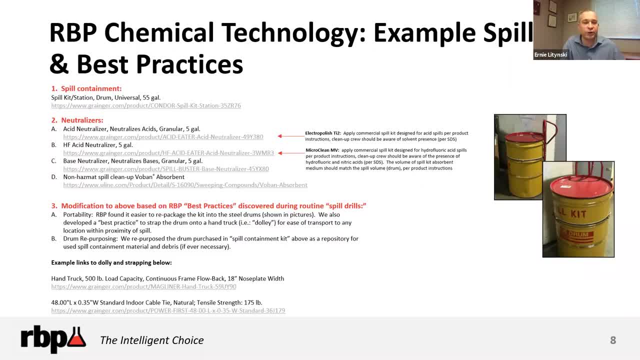 willing to translate, you know, and move forward to your organization as well. So with that again, HAZCOM, it's, it's, it's, it's a big piece and it's the fundamental portion of your program when working with chemistry. I'm fully dedicated right here. 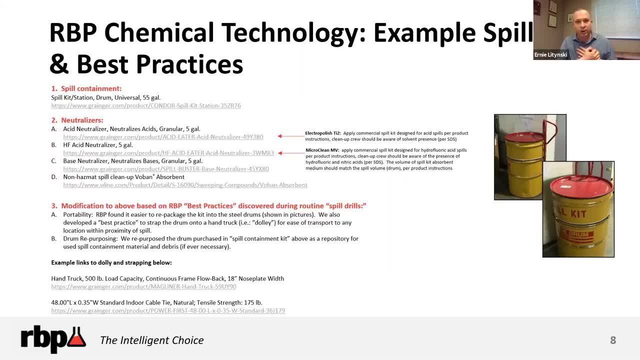 I'm telling you on this webinar. please pass it to your organization or your partners that you know we're willing to give you some considerations. Again, every plan's a little different but we're very willing to provide those best practices. so we don't reinvent the wheel. 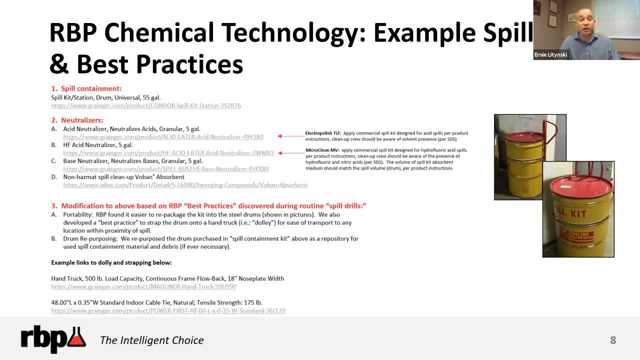 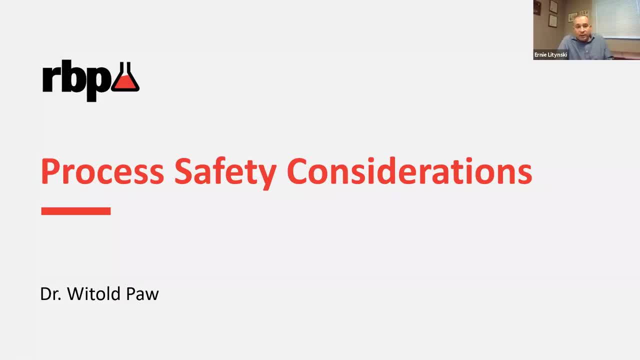 you know, in your organizations. So that concludes my piece of the briefing, And, and with that I'm going to, I'm going to pass on to Vitold here, Not you know to, to talk a little more. 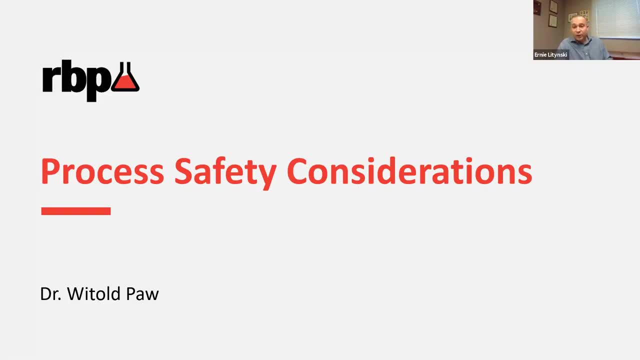 Vitold has been with RVPO for over half a decade and he is our R&D manager. He probably works with chemistry more than anybody here outside of our production folks And he's responsible for all our product lines here. And I'm proud to say that Vitold holds a PhD in chemistry, and we're proud. 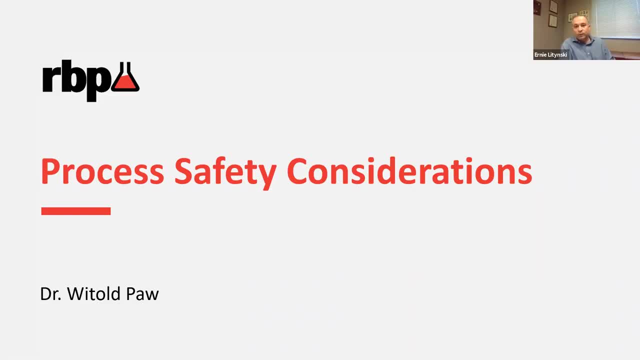 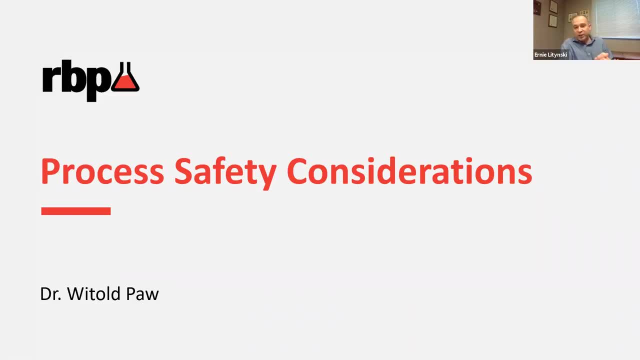 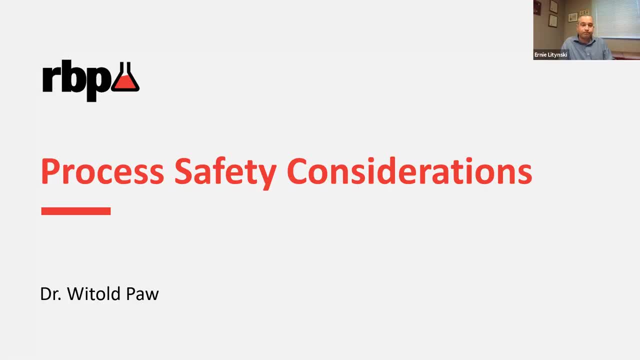 Vitold, I'm gonna pass it over to you at this point. Thank you, Oh, it looks like I was muted. Sorry again. Hello everyone. Both Ernie and Eric probably did not know that my other title is practical chemist. 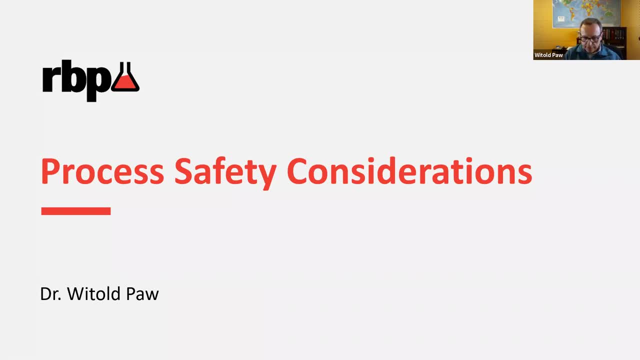 So I'm going to talk to you about some practical things that may be more relevant to your process area. I'm talking primarily, maybe, to process engineers, with whom I interact quite a bit, So we'll basically talk about those chemicals and hazards associated with them. 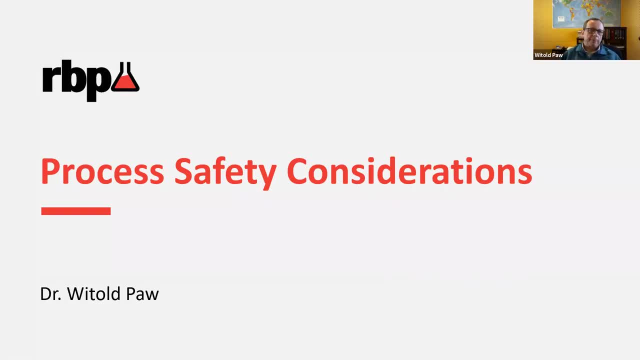 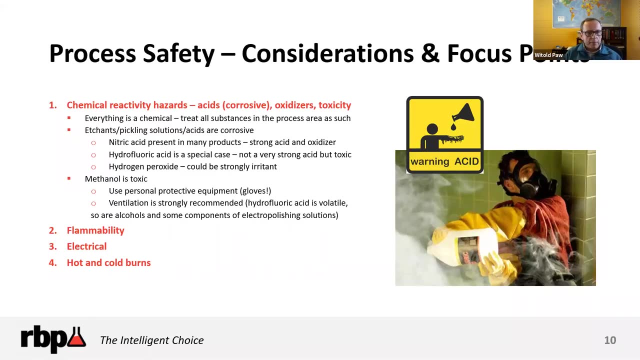 Next slide, please. So here they are In general. in addition to chemical hazards, there are also flammability, electrical and hot and cold burns. We talked about them on the next slide. But speaking about chemicals, there are a few of them that I think you already know that you should pay attention to. 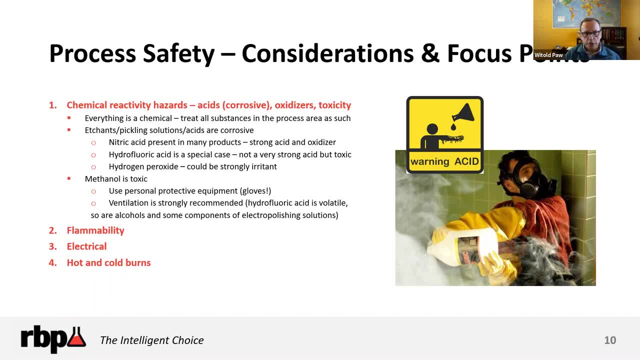 The types of hazards are: corrosive nature of acids- right, There are some oxidizers that you work with, And there is Some of them. some of the chemicals are toxic, So let's talk about some of those. I think nitric acid is present in many products, many products of ours. 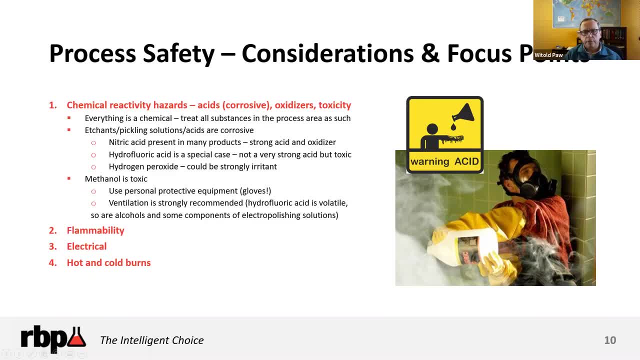 And it's present in your process area. It's a strong acid and oxidizer, So be careful with that. Another one, another acid, probably not as corrosive but probably more It's dangerous- which is hydrofluoric acid. 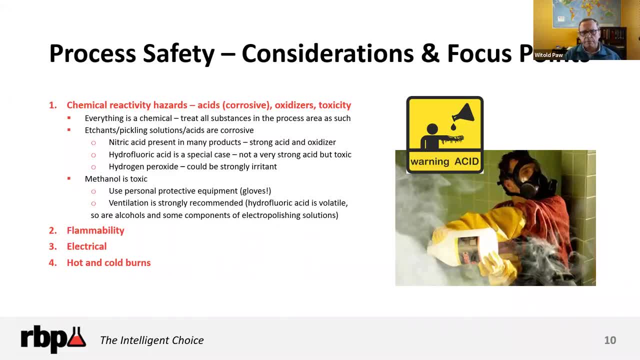 And here on the right hand side you have this great picture from the breaking, from Breaking Bad Jesse, dissolving a human body in hydrofluoric acid. So, yes, you can do that. So don't put your hand in in the beaker with hydrofluoric acid. 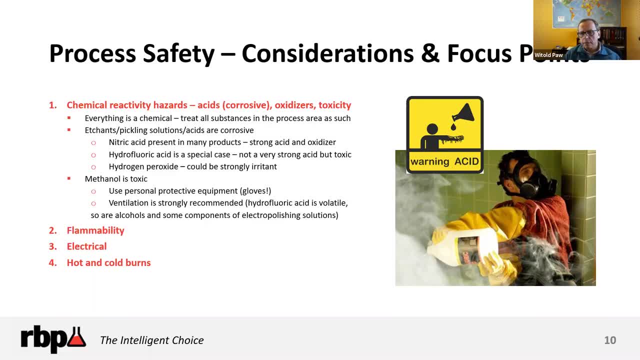 So the thing about hydrofluoric acid is that it's also volatile, So the toxicity comes also from inhalation, not necessarily from. So the toxicity comes also from inhalation, not necessarily from. So the toxicity comes also from inhalation, not necessarily from. 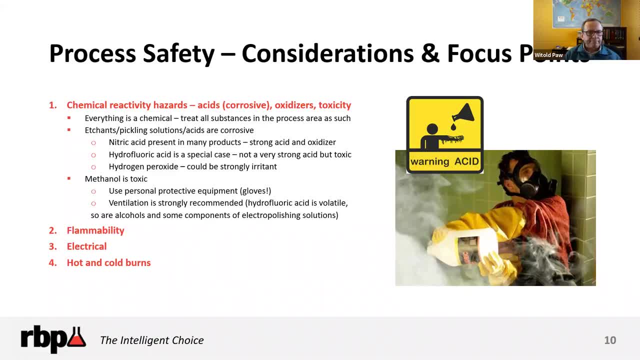 Contact right And also it's you know, if you get a burn on your on your skin, that the tissue will probably heal. The thing about hydrofluoric acid attacking bones is that you really have one set of bones and there is. your body will not repair those bones. 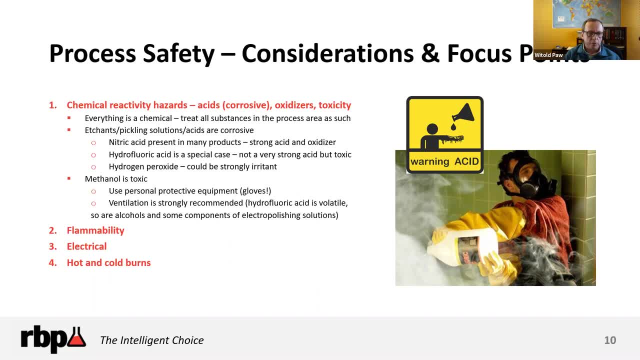 So that's, that's the bad thing. If you are, You know, exposed to to hydrofluoric acid, Yeah Yeah, If you are exposed to to hydrofluoric acid, be very careful about hydrofluoric acid. hydrogen peroxide, sometimes used as an oxidizer, can be strongly irritant to to to skin toxicity. 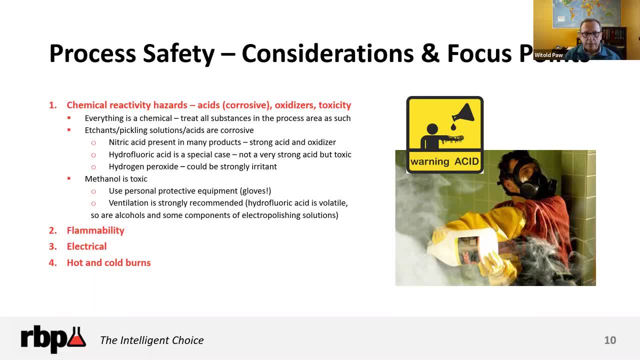 So, in addition to hydrofluoric acid, which is not just the acid, not just corrosive chemical, it's also toxic, There is also methanol, which is which has to be considered as a toxic And, again, it hadn't can be inhaled. 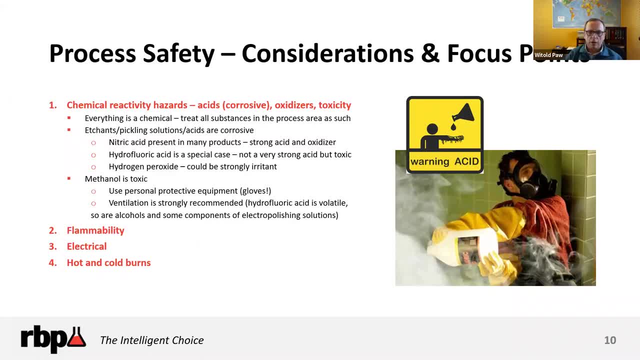 It's probably used as your rinses in in your EP station, So don't don't breathe that methanol. Ventilation is strongly recommended because of hydrofluoric acid and and and alcohols in your process area. Okay, 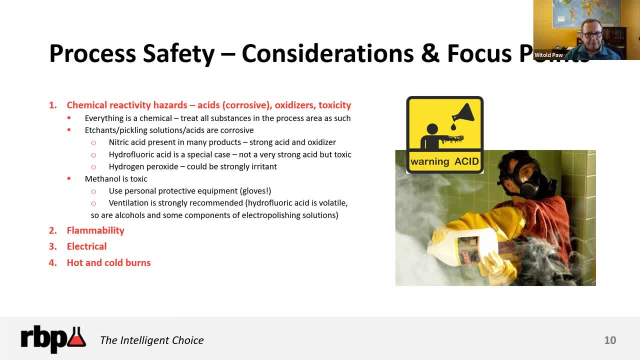 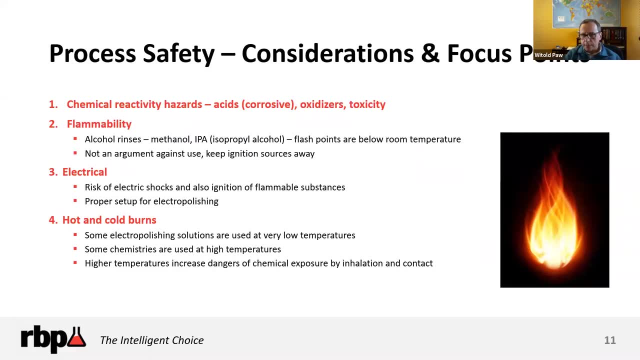 Let's talk about some other hazards On the next slide. Flammability: Some of the chemicals, some of the chemical products that you use are flammable, And it's you know. the thing about safety is normally use the farm with the flammability may never come into play. 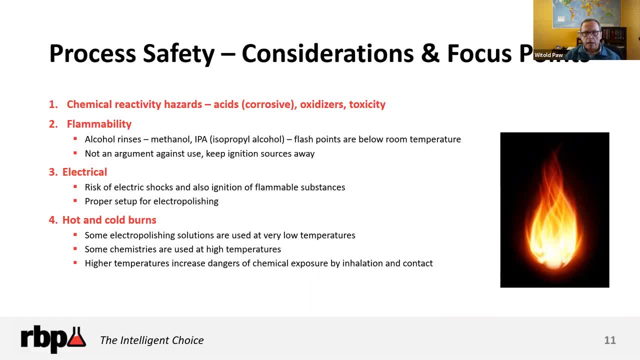 Right, But it's useful to remember that they are flammable chemicals and fires do happen Sometimes. they happen Not when you are working in your, in your home, In your area. they may can happen at night, especially if your your hot plates, you know, are left on and things like that. 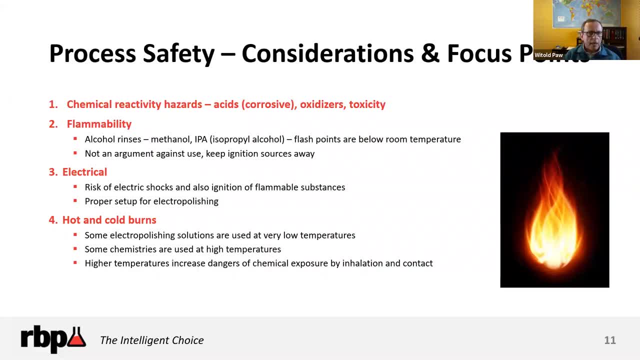 So there are also. it's important also to have those safety procedures, Something I forgot to mention. you want your process to be safe, effective and easy, right, And sometimes you may think about switching effective and safe, but but then many people say safety, safety first. 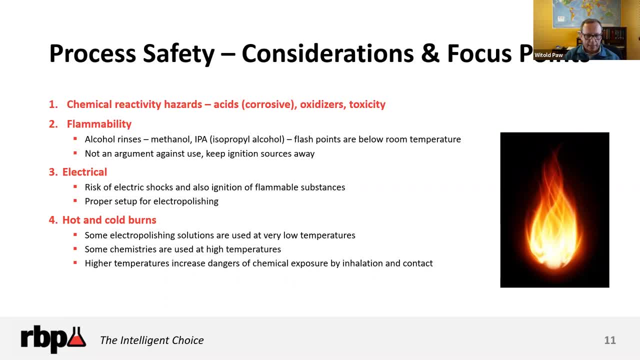 So These two are very important: safe and effective, easy. I pay attention to to ease of use, because when something is easy to use, it's also safer, right. So safe, effective, easy. Going back to flammability, of course this is not an argument against the use of flammable chemicals that they are flammable. 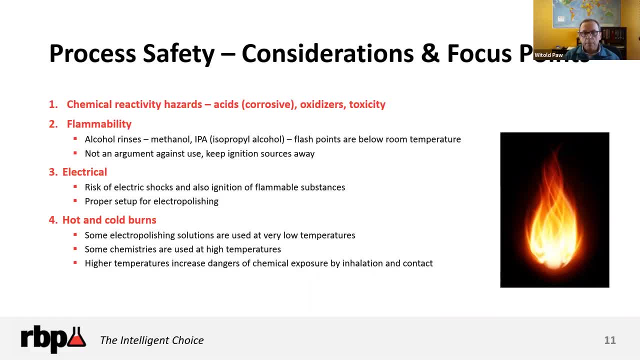 Just keep ignition sources away and just be mindful that they are flammable. They can happen, They can catch fire, they can burn Electrical safety. I'm sure your electrical folks at your facility will Make proper arrangements right. I think it is still important for you to remember that electric current may be a source of ignition of your flammable chemicals right. 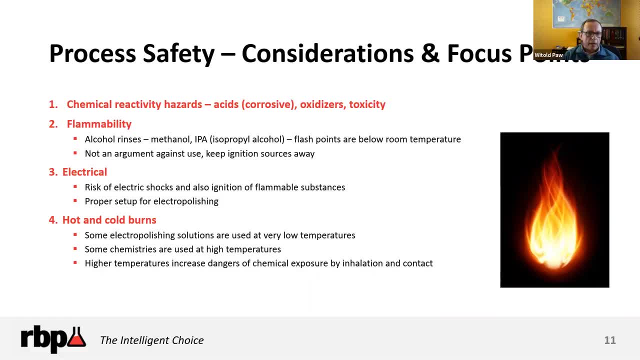 So this is really all new. So proper setup for electropolysis And avoid those ignition sparks from from your electrical equipment. I just want to also mention about hot and cold burns. some products that that you use are cold, like that standard sulfuric methanol electropolish and it's very cold so it can- can you know at least- irritate the tissue. 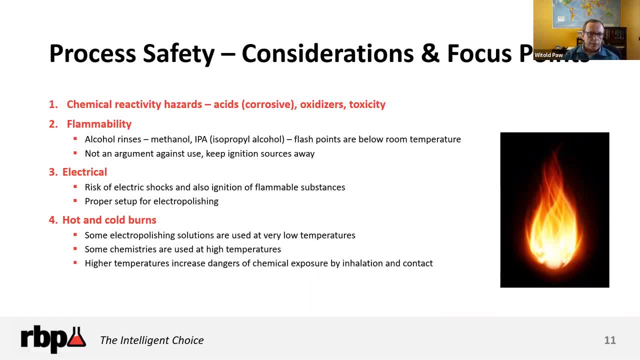 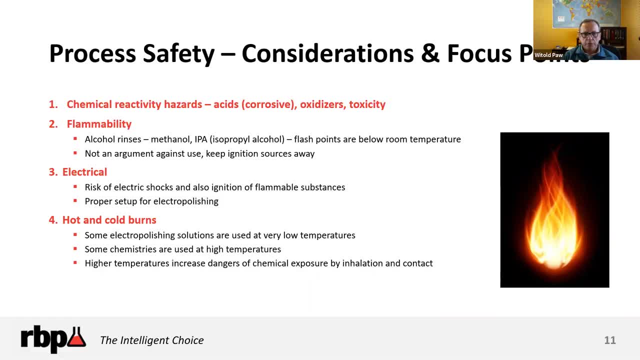 The temperature of this product that you're using to the oxidized to some high values. So high temperature and you know anything higher than 60 degrees Celsius is considered hot and you go to 80 degrees, it's really hot. One thing to remember also that 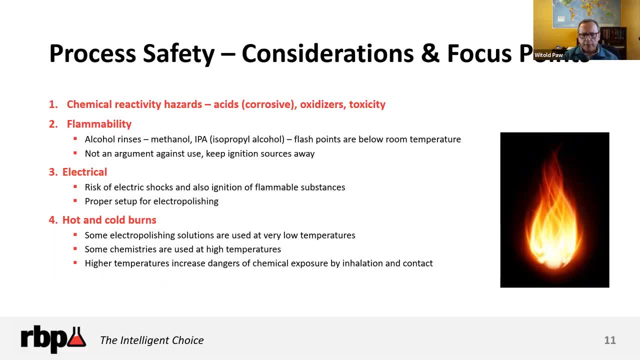 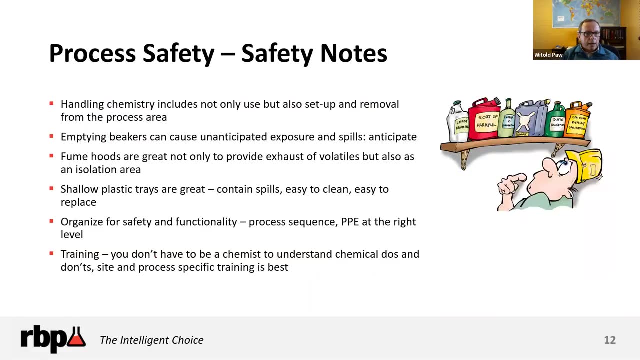 that higher temperatures increase dangers, right. That methanol is more volatile when warmer, or any alcohol is more volatile, right. And the acid when hot, it's much more corrosive. Be mindful of that. Okay, let's go to the next slide. 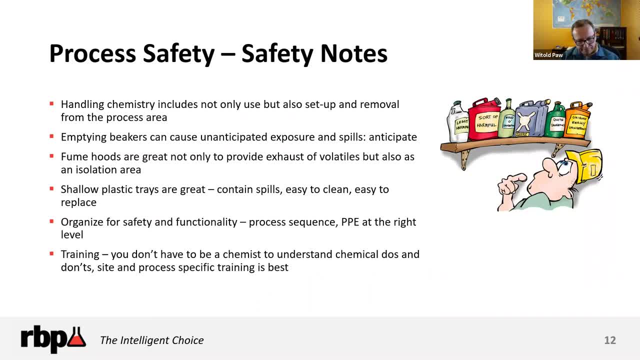 and talk about some practical stuff. I've seen many of those already in use at the customers that I visit, but there are some just good practices that are useful in the area. First-hand chemistry is not just using them in your process when you move your stand from one station to the other. 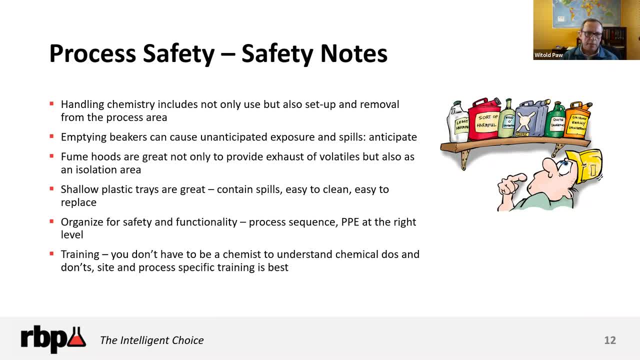 It's also how you prepare your setup and how you remove the setup, And that's really when your spills can happen. So what is the chance of your contact with a chemical if you are moving that stand from one beaker to the other? Probably negligible. 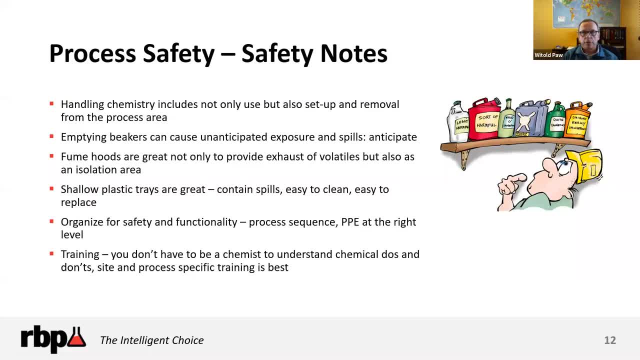 But when you replace the solution with a new one, that's when the spill can happen. So just be mindful of that. It's not just safety when everything is set up and ready to use. So emptying beakers can cause unanticipated exposure and spills. 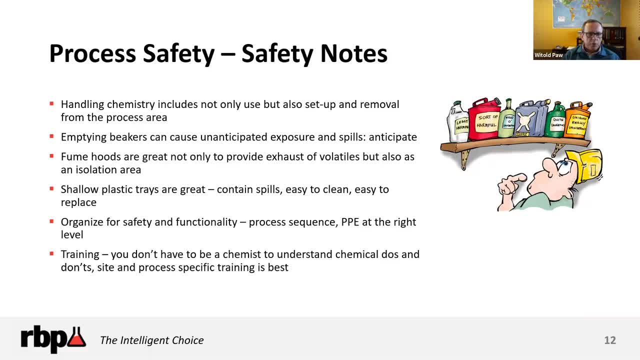 So you have to anticipate those situations. Fume hoods: they are great to provide exhaust, removal of volatiles, but they're also great as an isolation area just for yourself and also other people around in your facility. Shallow plastic trays are great to use. 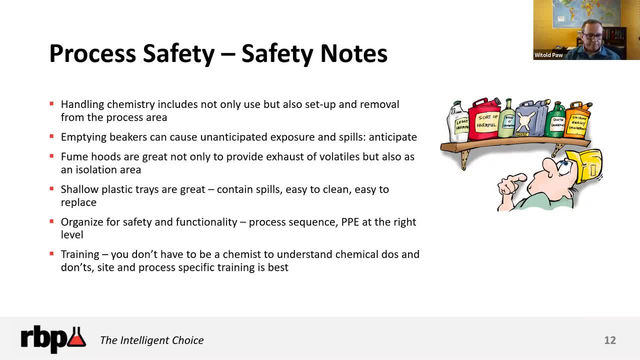 to contain spills, but also drips happen when you move the stand from one station area to the other. There is this drop that falls on the surface- And it's better if it falls on the surface of a plastic tray than somewhere else- and you clean it up. 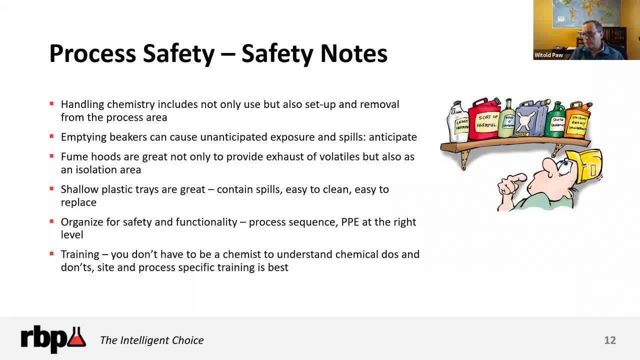 Organize for safety and functionality, Just if you move your stand from left to right, that's how it should kind of in your process area. That's how the stations should be organized, so that you don't have to move the stand from one station to the other. 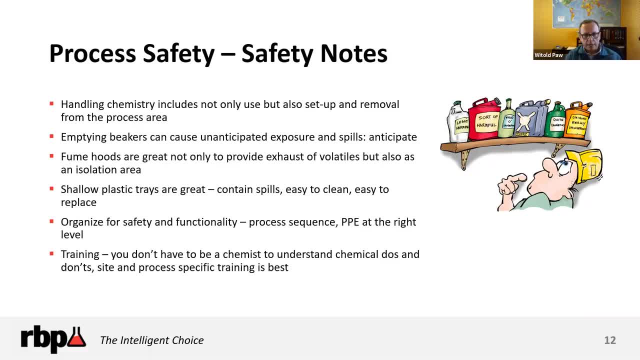 So that you don't have to move the stand from one station to the other, So that you don't have to move the part across a significant distance. Just it's easier that way and more practical Training. it's probably best to have somebody. 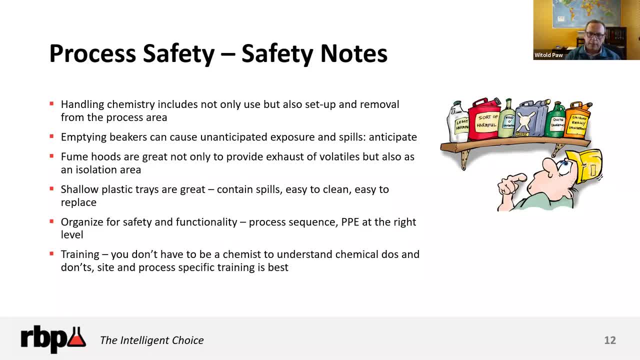 who has worked in the area to show you how it's done, what to look out for things like that. Again, I'm a practical chemist and I like those very practical approaches. I would like to attract your attention to this cartoon. 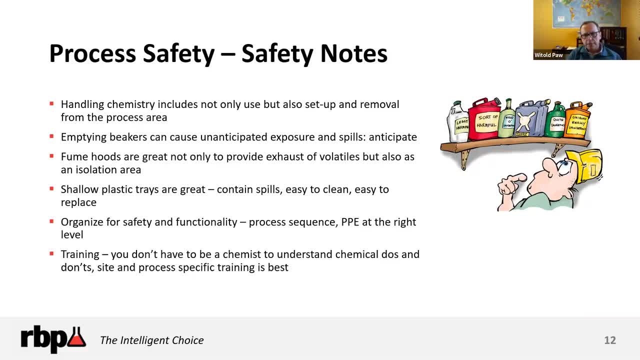 So it's kind of funny. but basically what it shows is there is a range of hazards associated with chemicals. There are least harmful on the left-hand side And I bet you haven't seen those. Really what, oh my gosh, really dangerous. 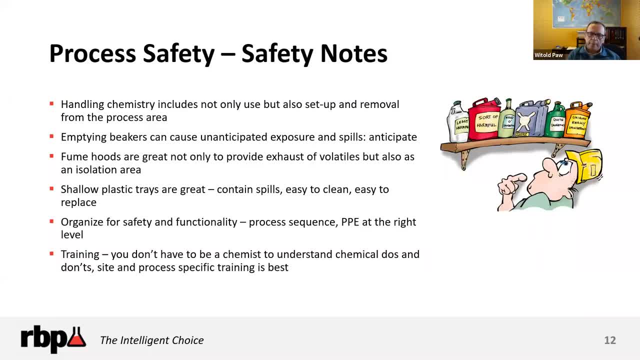 I think we probably, when we sell our chemical products to you, we probably have products from the left-hand side to like, in the middle of the shelf, Some more hazards, Some more hazardous than the other. So if we go to when we go to the next slide, 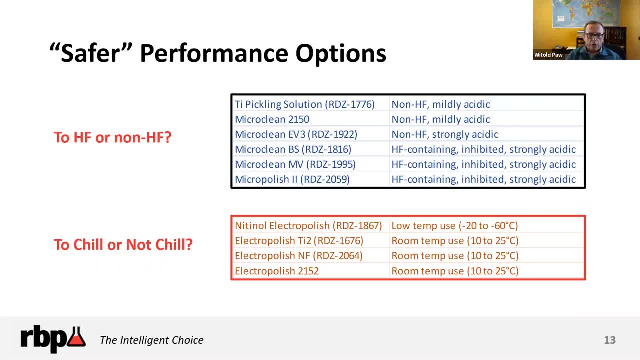 I will maybe mention some of those. So first of all, to deoxidize, for example, nitinol. I'm showing a bunch of nitinol deoxidizing products. It's best to think first about those non-HF deoxidizers. 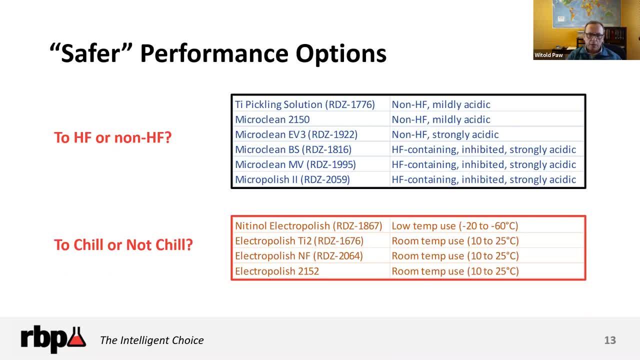 because they may work just fine for you. So you don't have to go to the the chemicals which which up the level of of hazard by by having hydrofluoric acid containing them. So micro, micro clean EV3 may work just fine. 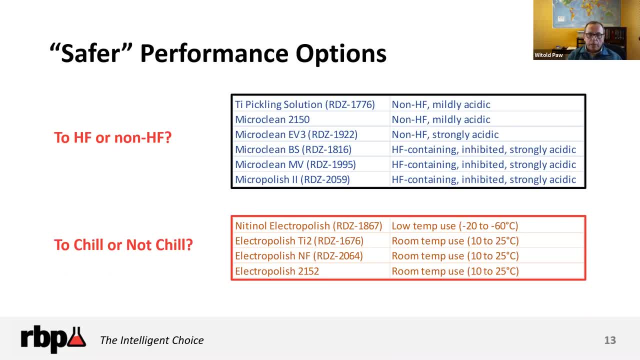 to deoxidize nitinol. So we, in many cases, those safer chemicals have equivalent performance or they would. as I said they would, they would do the job. So we have that offering to you and we highly recommend it. 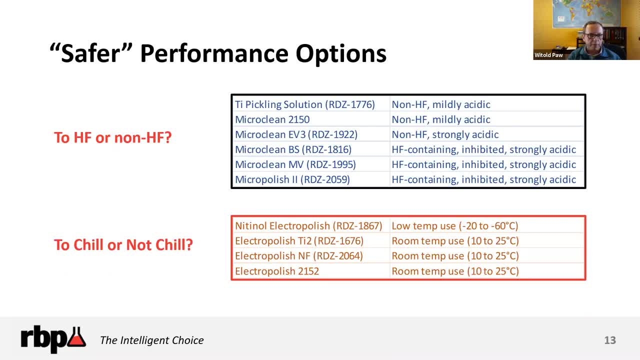 So we have that offering to you and we highly recommend it. So we have that offering to you and we highly recommend it. I certainly recommend you to do safer chemicals first. Sometimes, of course, it's not possible. You may have to use, for example, microc. � 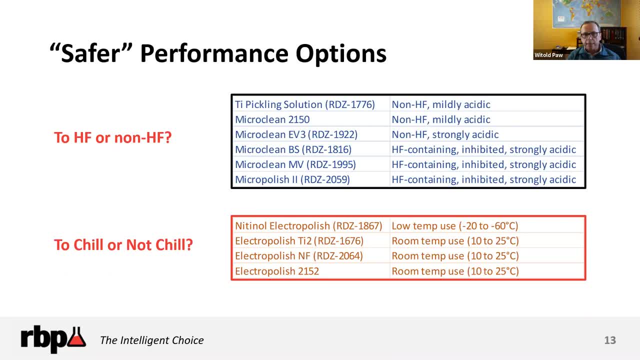 And of course, I don't want to say that it's a dangerous product. right, It's just the SDS, for the product is a little bit different And of course, you should reviews SDS carefully before you use it. As far as electropolishes, I am change. well, yeah, yeah. 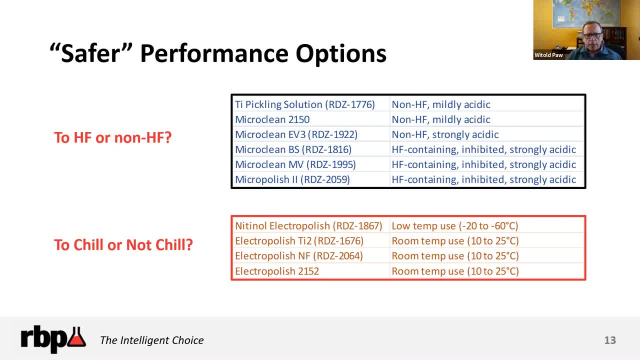 are concerned, this is more about ease of use, which has practical and safety implications. We do provide nitro electropolish to our customers, which is that electropolish solution that needs to be used cold, very cold, But we know that there are equivalent products of products of. 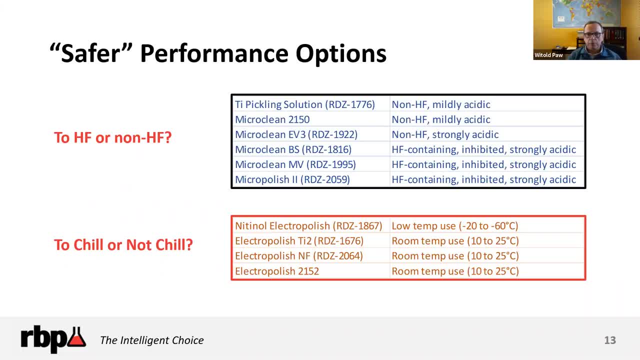 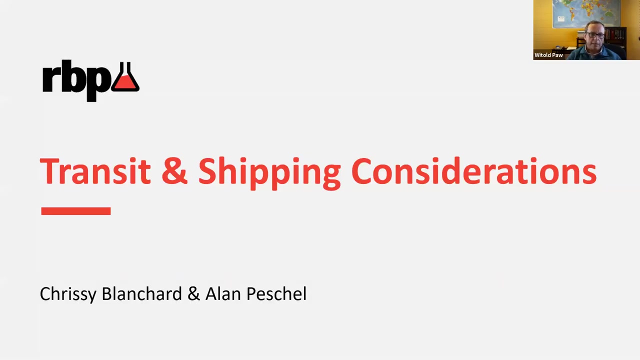 equivalent performance that can be used at room temperature. It's just faster and safer to use those, so we highly recommend those for you to consider. I think that may be it. Can we check the next slide? Yes, so next you will hear from Chrissy Blanchard and Alan Peschel about transit and shipping. 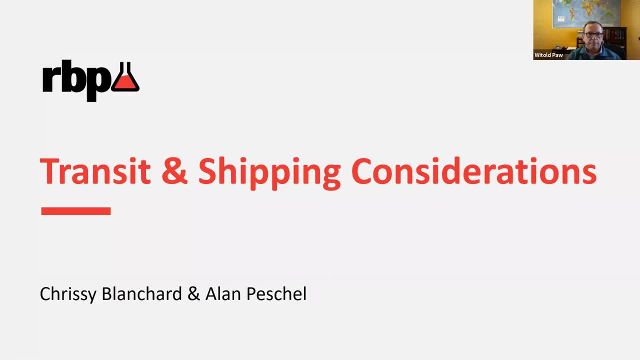 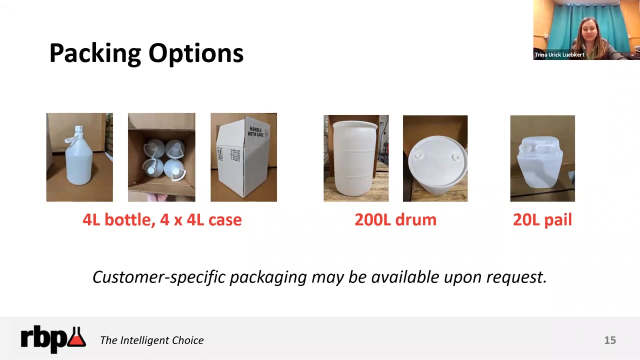 Thank you, Vitold. I will be talking about RBP's transit and shipping considerations of our chemistry, whether hazardous or not. Chrissy, you're on mute. Thank you, Sorry about that everybody. So RBP's chemistry is offered in three standard pack sizes. We have our four-liter bottle. 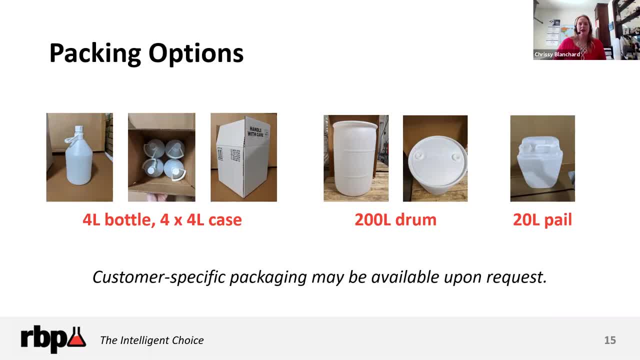 which you can see on this photo. We can send them individually or four bottles to a case. We also offer the chemistry all the way up to a 200-liter drum and a 20-liter pail. All of our packaging is UN certified, meaning that it is designed and approved to safely contain. 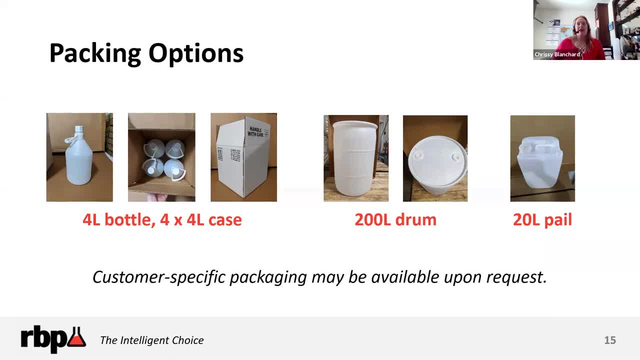 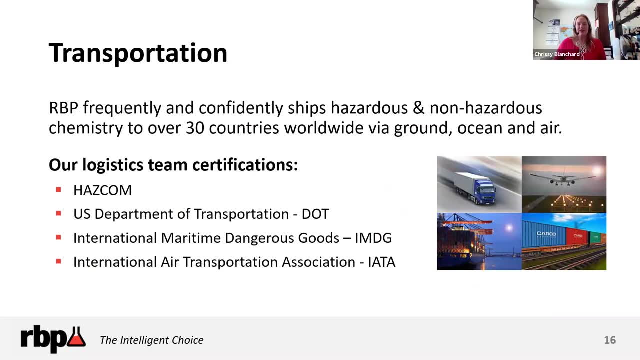 dangerous goods under normal conditions of transport. This means that it is designed and approved to safely contain dangerous goods under normal conditions of transport, And customer specific packaging may be available upon request. RBP frequently sends hazardous and non-hazardous chemistry globally to over 30 countries via ground. 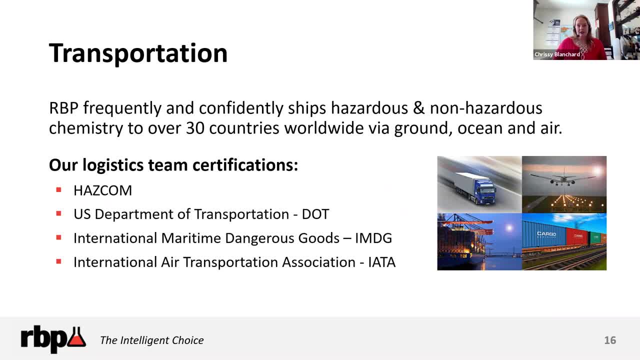 ocean and air transportation To do so. our logistics team has certifications in these different areas. Haz, foster care or Human Bulletproof Commerce can be sent on a container successfully. This is the area that Ernie talked about earlier. To repatriatewarrior, local commerce lines and non-coronavirus supplies, smile provides a local one-day over the world cost to bed as are f summoning and sleep largestー. 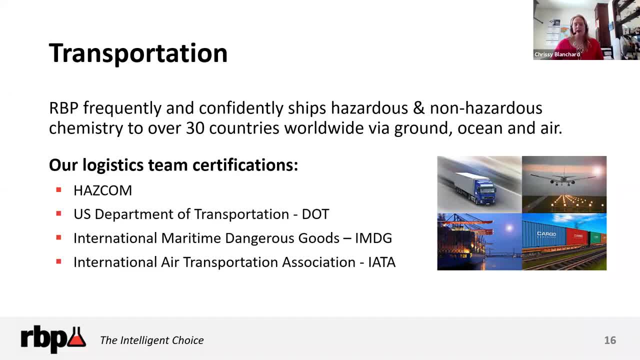 a last-minute access to the energy testing facilities. services anddır fucked. passengers from over 30 countries from an area close to us have a special of certain speedoudl hazardous communication training DOT. this is the US Department of Transportation and this 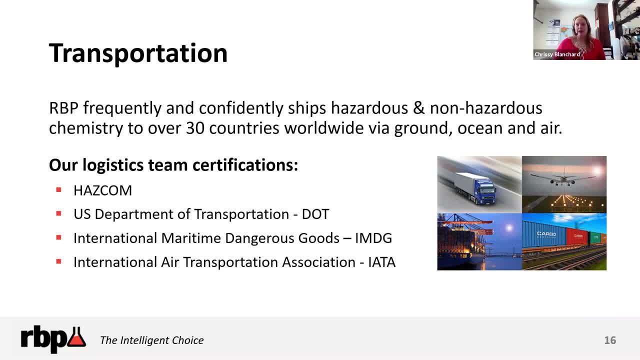 regulates our ground transportation for sending hazmats. The IMDG is the International Marine Dangerous Goods- This is for when we are looking to send our chemistry overseas. And lastly is IATA, and that's the International Air Transportation Association, and this defines the regulations. 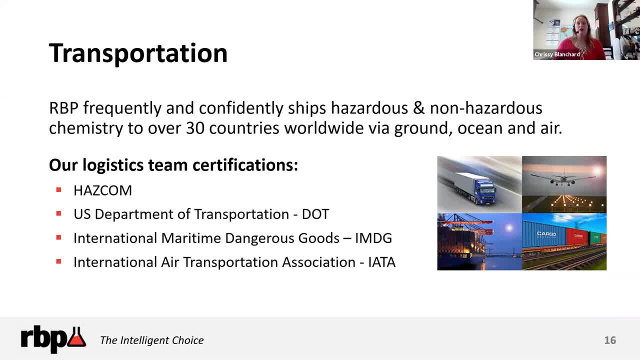 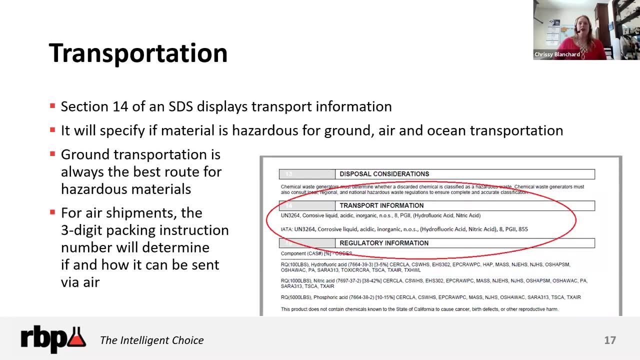 required for sending products via air, And so, as you can see, we've got many different considerations to put into place when we need to send our goods to you. Section 14 of the SDS, again talked about earlier, this section outlines transport information If a product was non-hazardous and there was no. 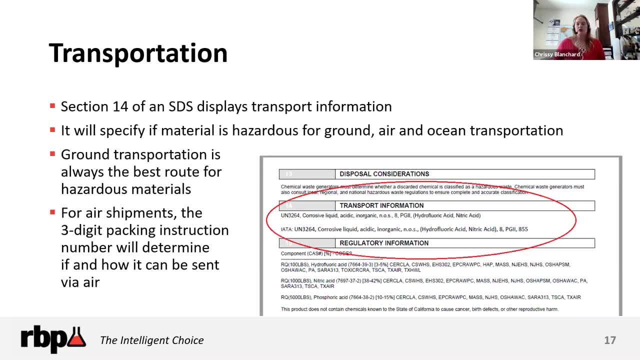 regulations to put into consideration. it would simply say, not restricted for ground, ocean and air transport, And, as you can see, ground transportation is going to be the best route for sending the hazardous materials. However, many of the chemicals that we provide are hazmats, And so here you're going to find 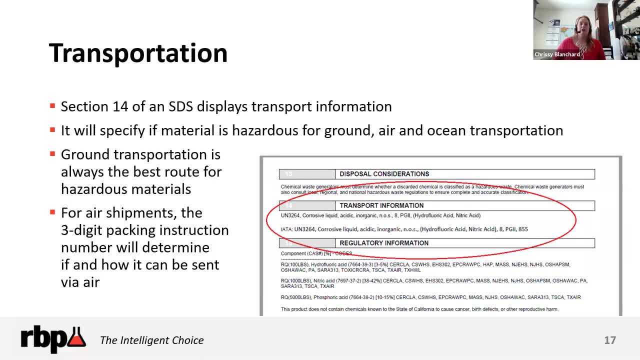 that hazardous information. Ground transportation is always going to be your best route for handling the or for sending the hazardous materials, and, of course, domestically. that's usually not a problem, but many of our customers do happen to be overseas, So we have to put in consideration: what are the regulations that we need to send? 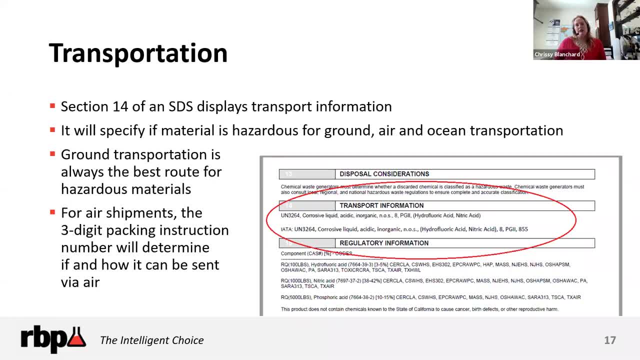 to know about and to plan for for sending via air and ocean transportation. And on the SDS, section 14,, again, the IATA will be right there. We like to look immediately at the three-digit packing instruction when we do need to send air, and this will help us determine. 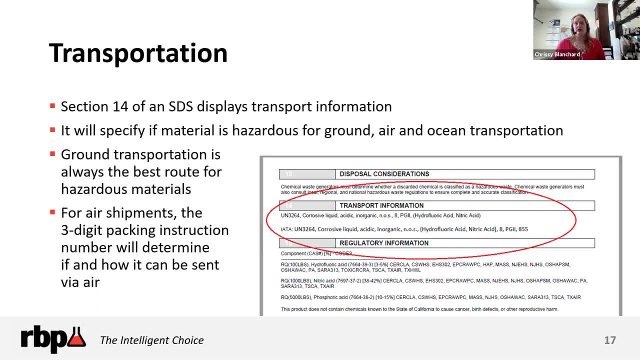 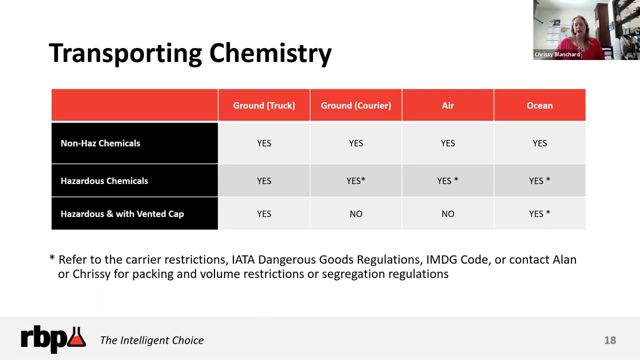 what specific packaging that we are restricted to. But pretty much most of our products can go any means of transportation. This next slide is a chart. It's an at-a-glance look at our options when transporting chemistry. Obviously the non-hazardous has the least amount of restrictions. 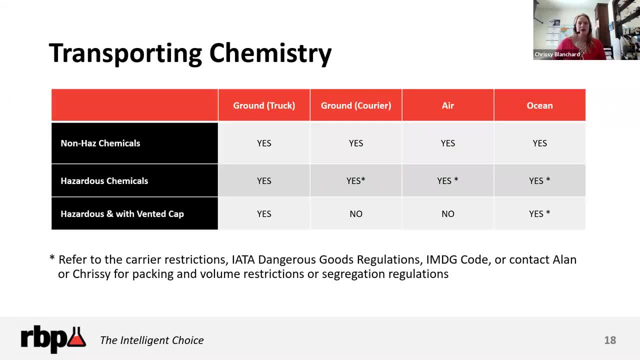 Hazardous chemicals will have some restrictions which we are certified to work with And some products do have a vented cap which we have. Again, you can refer to the DOT, IATA or IMDG regulations for the volume restrictions. 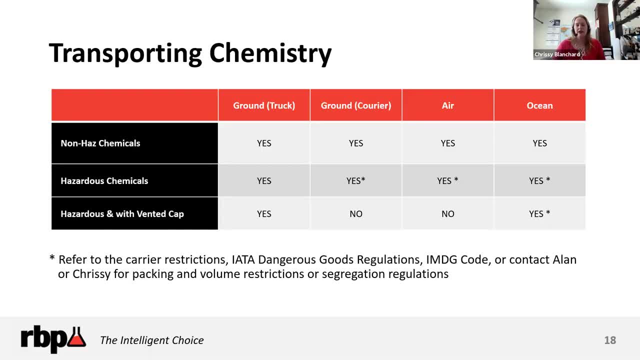 any segregation restrictions that are required for sending material, And if that's not something that your team is qualified to do, you can certainly call RBP, speak to myself or Alan and we will surely assist in figuring out the best way to get our chemistry into your hands. 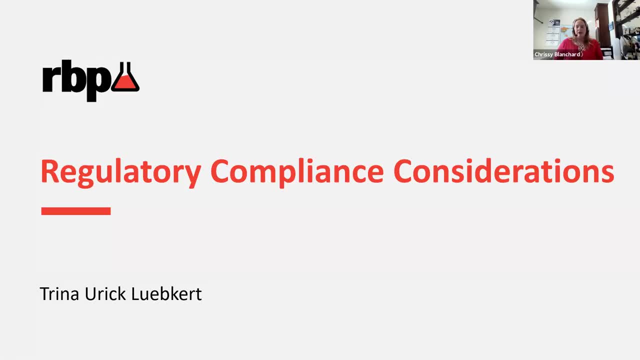 Now that we've shown you the items to consider when shipping hazardous and non-hazardous, our final presenter today will cover regulatory compliance consideration. That will be Trina Ewek-Lukburt. Trina has been at RBP for five years. She's our senior chemist in our product. 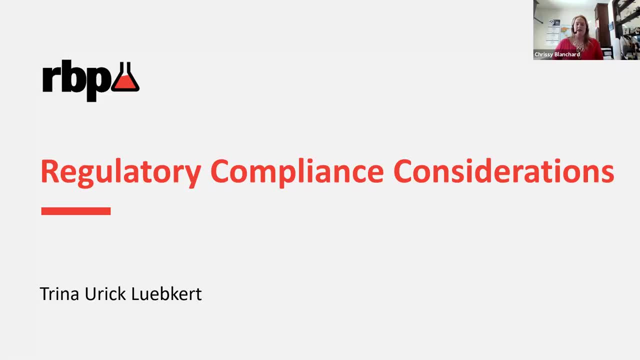 development team, as well as RBP's chemical compliance subject matter experts. Trina Ewek- Thank you, Chrissy. Chrissy Ewek- Thank you, Trina Ewek-. Thank you, Trina Ewek- As she said, I will be speaking about regulatory compliance considerations. 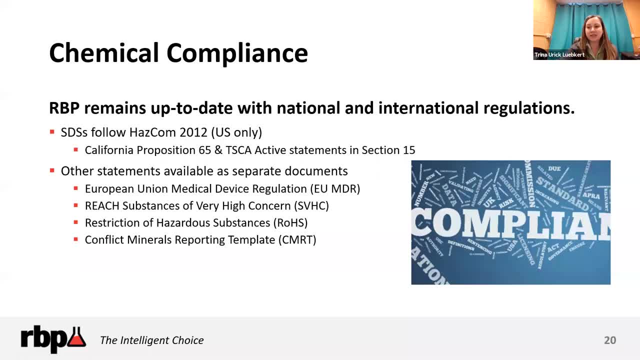 May I have the next slide please? RBP remains up to date in national and international regulations and we communicate this to our customers via SDSs, as we have already touched on today, And some things you'll find on an SDS already are a California Proposition 65 statement. 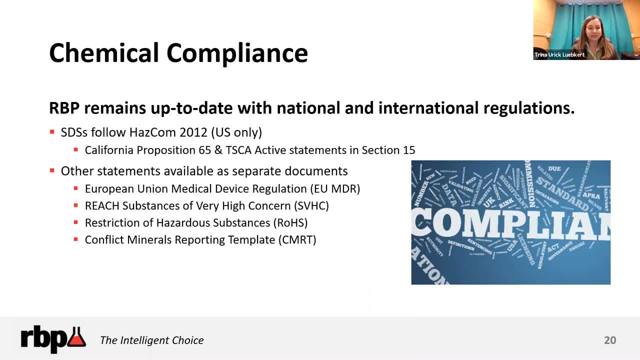 and a TSCA active statement. You can find these in Section 15.. Trina Ewek- Now, if you have customer requests, such as EU MDR or a European Union medical device regulation, a REACH SVHC or a ROSE or CMRT request, come in, you're going to always. 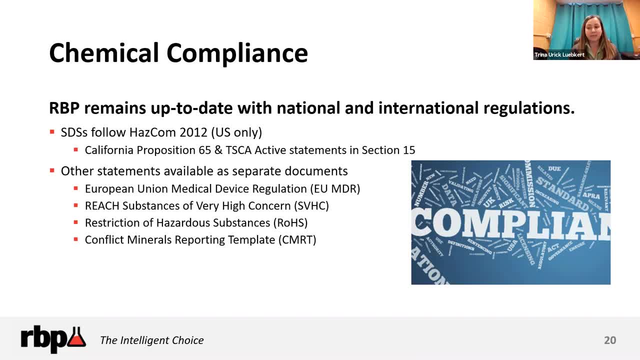 contact RBP directly for these statements. We provide them on request. and I think that's it, Trina Ewek-. That concludes my portion, Trina Ewek-. My portion, Trina Ewek- So I would like to hand it back over to our moderator. Thank you. 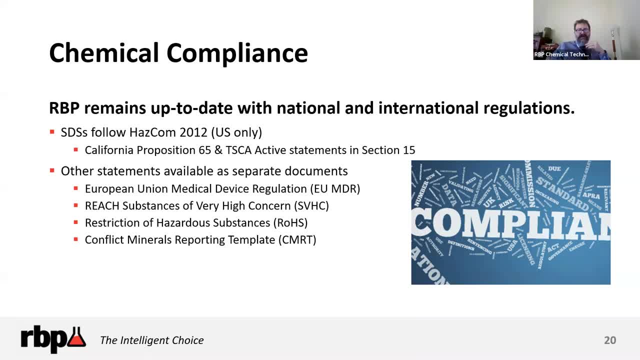 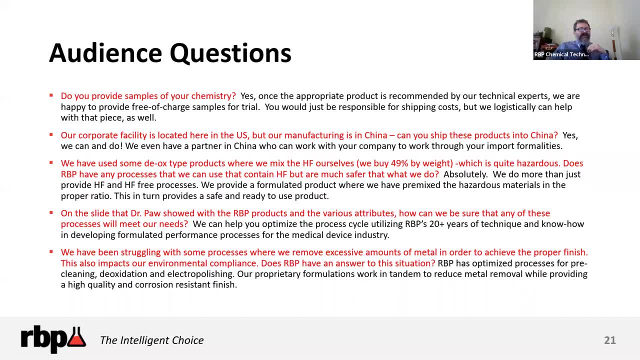 RBP- All right, Thank you very much, Trina. This is the part of the show where you can ask questions. We do have a couple of frequently asked questions that we're going to go through To ask a question, like I said earlier, just click. 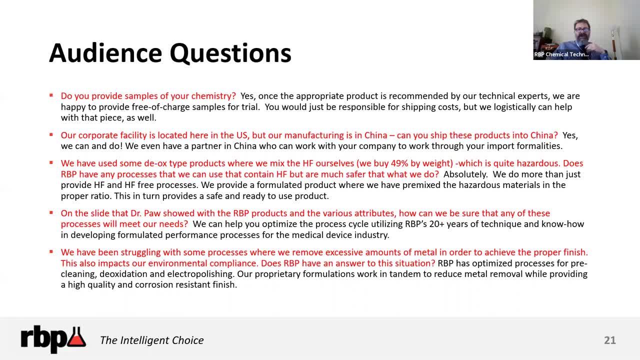 on the Q&A on your webinar controls, Or if you see a button that says raise your hand, you can do that and I can ask you a question. If you don't have a Q&A, you can use the Q&A button on your 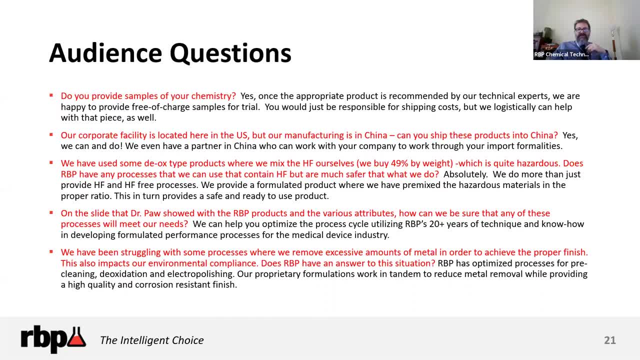 webinar and I can turn your microphone on and you can ask the question verbally. We recommend writing the question down, though. It's just a lot easier. First of all, a question we get all the time: Do you provide samples of your chemistry? 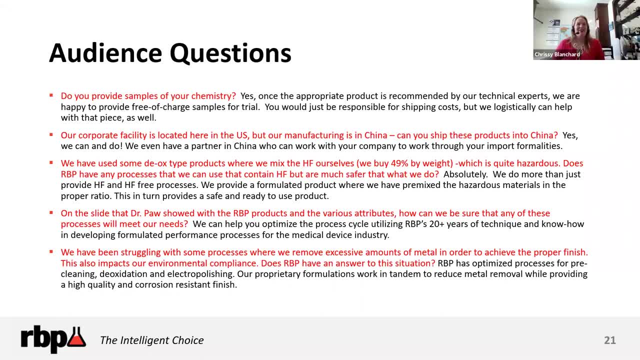 I'm going to throw that one to you, Chrissy. Chrissy Teigenbaum- I will definitely take that one over. So yes, we do provide free of charge samples. It's a process that we have to qualify to make sure that the proper product is being recommended by our technical experts. 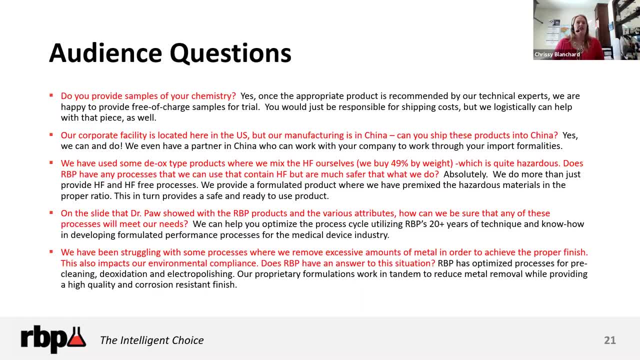 But you would just be responsible for shipping costs, however, but we will logistically take care of that piece as well, if you need that assistance. Okay, I'm going to keep you on the microphone for just a second here, because I think the next one also would go to you. Our corporate facility is located here in the US. 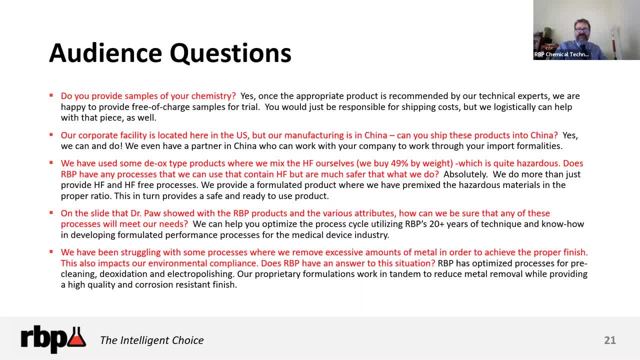 but we also have manufacturing in China. Can we ship these products and can we ship these products to China? Chrissy Teigenbaum- Yes, that is a very common question. China is often seen as having trade barriers for getting chemicals into the country, especially hazmat. 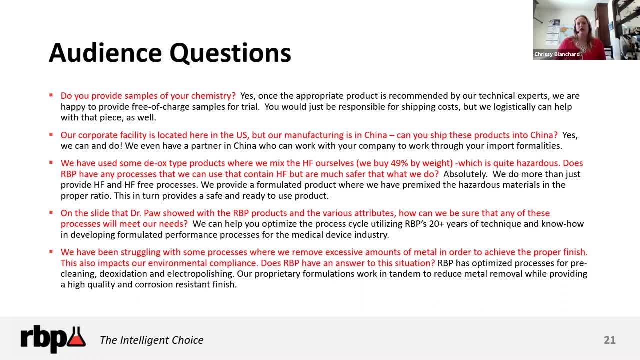 And we have overcome that by building a relationship with a partner in China who can work with your company to go through those import formalities bringing in the dangerous goods and whatnot. So absolutely do contact us if you're looking to send the products there. 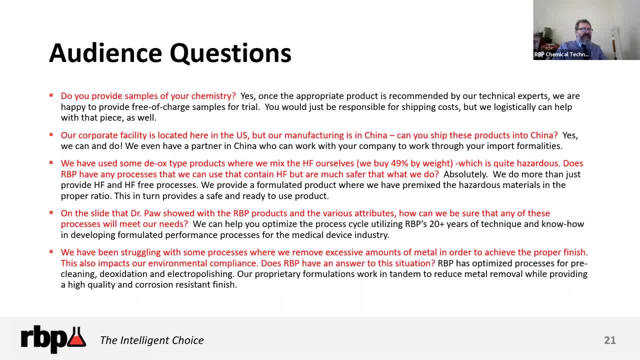 All right, Perfect. Thank you, Chrissy. Next question is: let's see, we have used some deox type products where we mix the hydrofluoric ourselves And you can probably see, as I say, we buy 49% by weight. 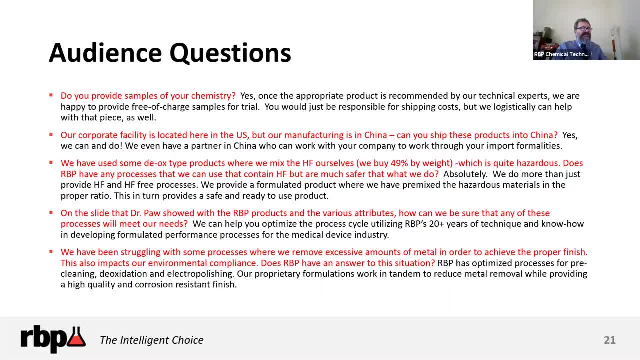 which is quite hazardous. Does RVP have any processes that we can use that contain hydrofluoric but are much safer than what we do? I'm not going to answer that one, but sorry, let's see here I'm going to toss that one over to Vitold or Mike Carano. 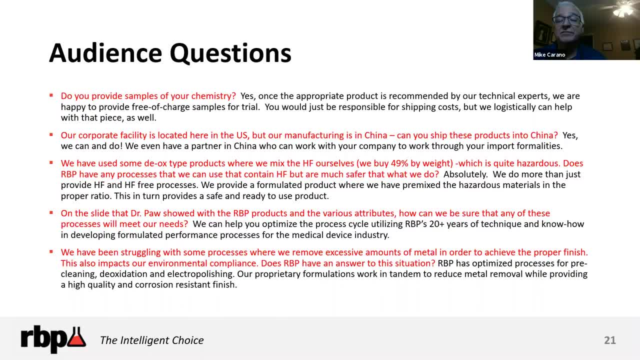 Vito Carano- I'll take that first and then Vitold can add to that. But the answer is correct. as you saw in Dr Pav's presentation: 49% by weight. hydrofluoric acid is extremely hazardous, But what we do is we have hydrofluoric acid processes here among. 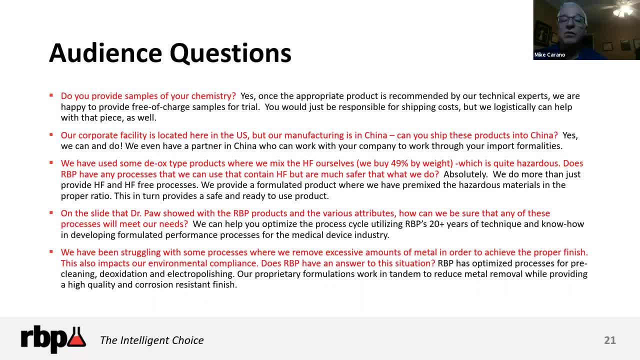 But we and RBP, as Ernie had said, we are a world-class manufacturer. We understand, we have trained personnel to understand how to handle chemistry safely, to not only protect the people who work with the chemistry, but also to ensure that we. 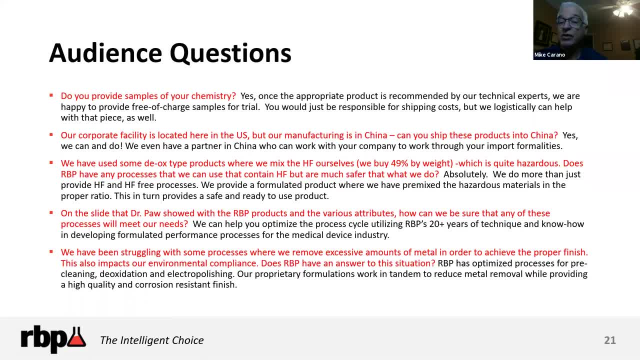 are handling the chemistry safely within the workplace and in our environment. With that said, we are skilled at mixing and handling these types of chemicals. Now, from our customer standpoint, if they have a plant that they're building for a medical device and it requires a hydrofluoric acid homebrew mix, that is very dangerous because 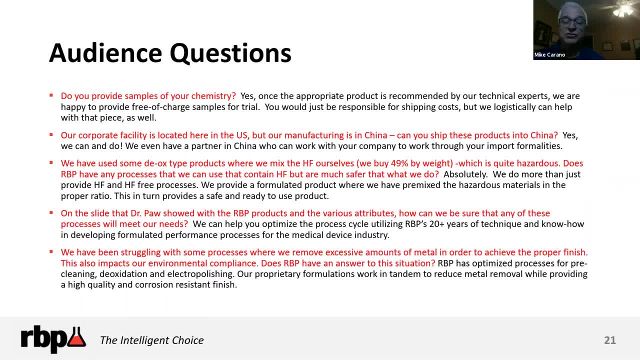 you are now asking your internal people, who are mostly metallurgists or designers or people who run the product down the line, to also handle 49% hydrofluoric acid and mix it. That is very dangerous. We have processes that contain hydrofluoric, but we've already done the mixing for you. 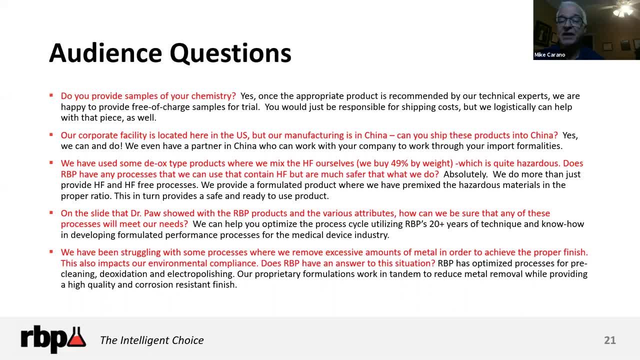 We've removed the exotherm, We've removed the danger And yet hydrofluoric acid, even at lower concentrations, is a hazardous material. But we've already brought that, taken that risk out of the process for you And we have a multiple portfolio selection of hydrofluoric acid-based processes that 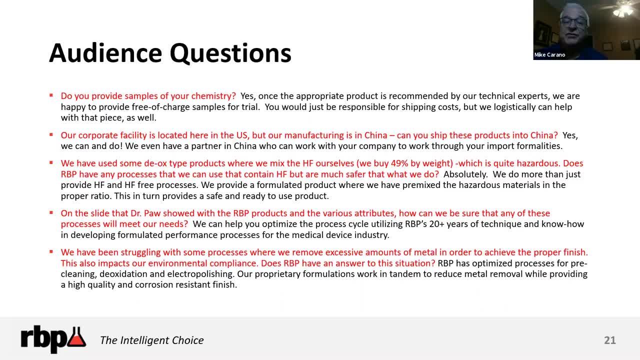 will meet your needs. That's another thing We also do: Toll blending. We are, as I said, a world-class manufacturer And if you have a formula that you like, that you've used for many years and it's a legacy- 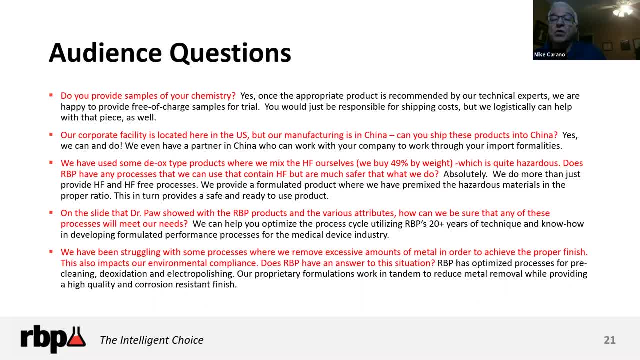 product that you can't change the formula. we can mix that formula for you under your requirements and certainly under an NMDA, So we can take the risk away from you that way as well. Okay, Vito, What do you have to add to that? 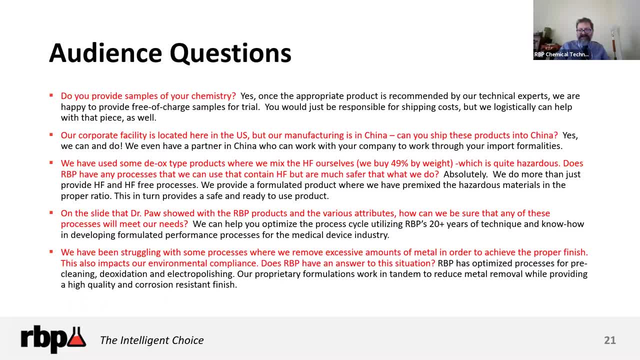 Or Ernie, you're on the microphone, So if you'd like to add something, Hey. just to mimic Mike's point: Look, at the end of the day, with things like HF, I'm not worried about a growth spill. 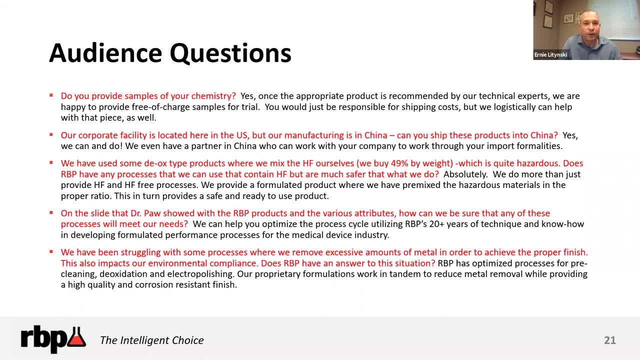 We'll see a growth spill. I'm worried about droplets of hydrofluoric acid, And that's more dangerous to me many times. So it's those types of scenarios that Vito talked about a little with what you have in process. 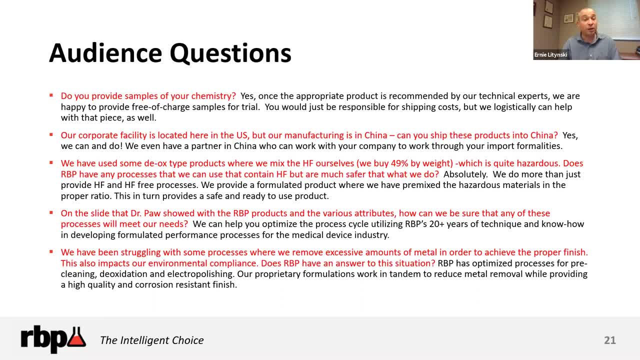 You know, and spill kits and so forth, because it's the little droplets that are going to get you And again, a growth spill. you'll see, You'll take the call to action. But on things like this, when you start talking with HF, you know pre-mixing it or using 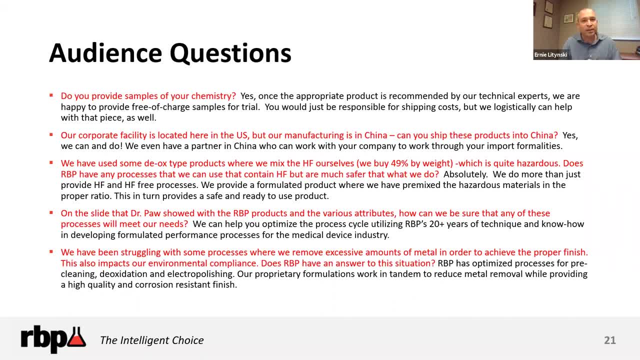 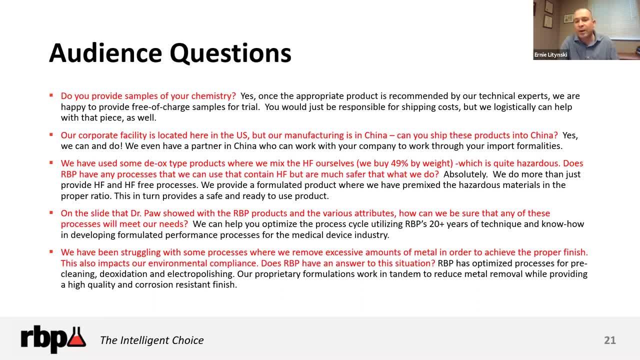 and have those mechanisms. So, Mike, that was a good adder, you know, or a correction. Hopefully this was a good adder to it, but just something to think about. going back to what Vito was talking about as well, with chemistry in process, especially when you're talking, 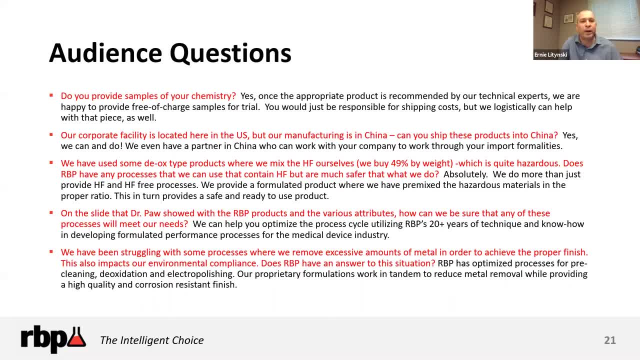 about something like as dangerous as you know, hydrofluoric 49% by weight product. Thank you, Yeah, this is a good point to to to dovetail to what Ernie just said about the droplets and the things. you don't see, the fumes, particularly when you're mixing multiple chemicals. 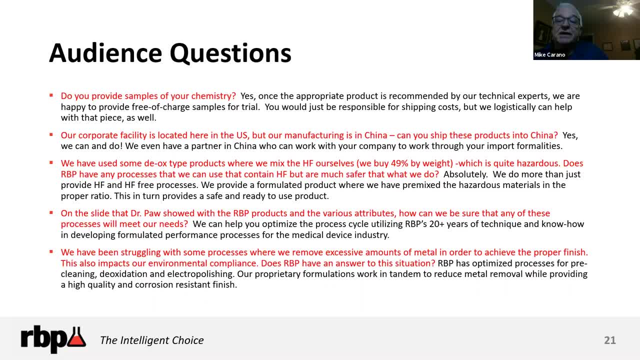 together on your own from concentrates when you're not used to doing that. Yeah, this Your health and safety folks within your company are going to be very worried about this. but so please make them understand before they say, oh, we don't want hydrofluoric acid in the. 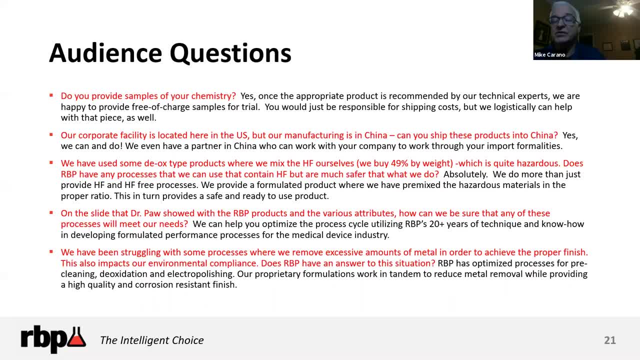 facility. Make sure that they understand we can help you take the risk away from that if you're mixing up your own. And, of course, the fact that we also have the non-hydrofluoric processes as well, which are gaining a lot of traction here for RPP- And again this is RPP's response to 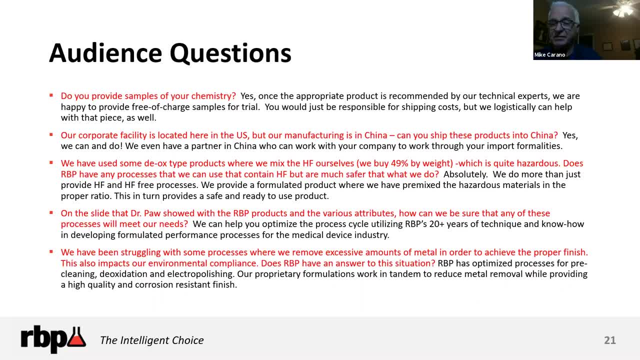 our customer needs. It's a response to the voice of the customer. We're an environmental company. individual as an environmental, health and safety person within that organization says: man, is there anything else we can do? What does RPP have? Well, RPP has an extensive portfolio. 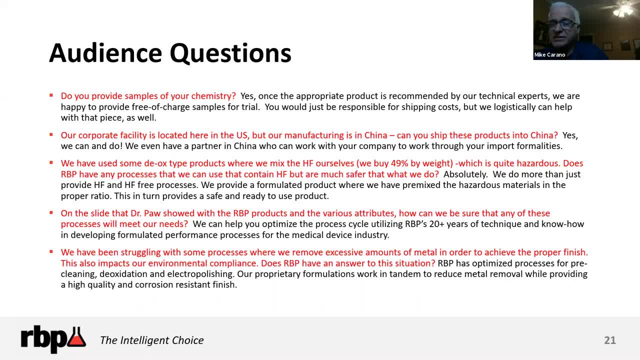 of formulated performance processes, cleaners, deoxidizers, electropolishes and chemical polishes that will meet your needs, not just for nitinol, but for cobalt, chrome, stainless steel and various titanium. So I just wanted to make sure you understood that, And we work with you as a partner. We are 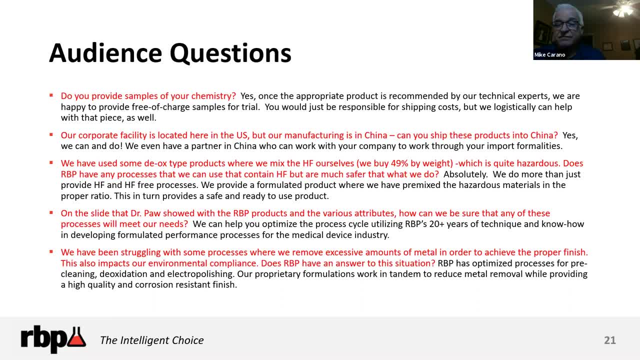 subject matter experts and we provide consultative selling, basically to help you meet your needs, recognizing that you all have something different maybe in your process. whether it's heat treating, laser cutting, whether it's an argon, oxygen, nitrogen, all of those things can affect the 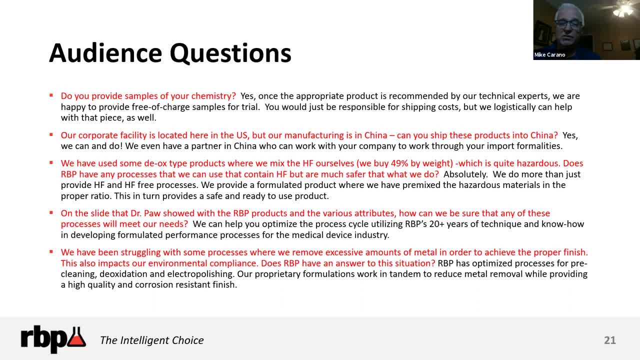 performance, how these chemicals work. Well, we have the answers for you. Yeah, Mike, that was good. I think we had four and five there too with that. So some of the questions. All right. We told his microphone on for a long time now, So I'm going to give him a moment to. 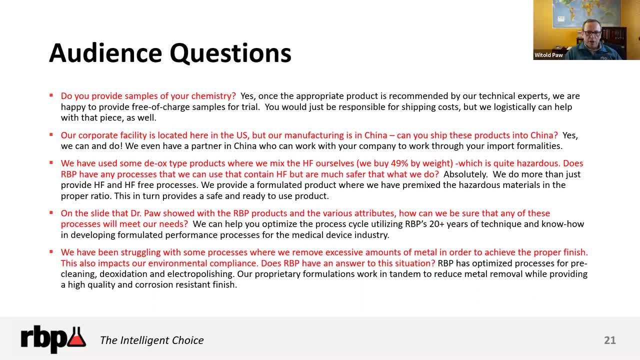 chat about this as well. I'm not sure how much I have to add here. You know, the situation is often that you may or may not use hydrofluoric acid, And if you can, because this is a company- we may be actually your good option, because we offer those that do not contain HF Hydrofluoric. 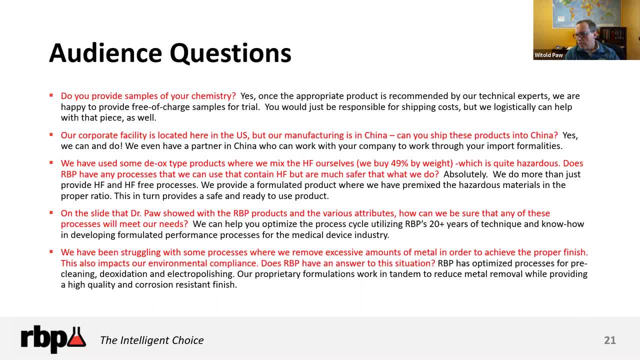 acid is quite popular out there. You know that's what people know that should be used to process many of those metals. But we do have those alternatives And when we select the product for your process, we always turn first to those that do not contain HF, because it's just safe. 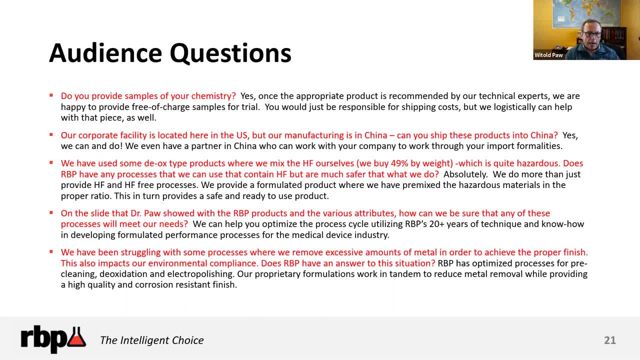 It's better And you know that. our products that we have dedicated for these processes, you know they contain hydrofluoric acid. But if you don't handle the 49% yourself, the danger is actually much lower to you because it's related. The danger is related to concentration of. HF in the product And many of the products work at only you know 2%- and you probably know this 2%, 3% of hydrofluoric acid in the product. The difficult part may be what else to put in that. 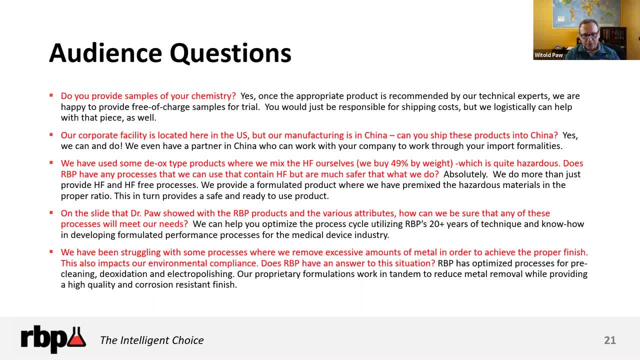 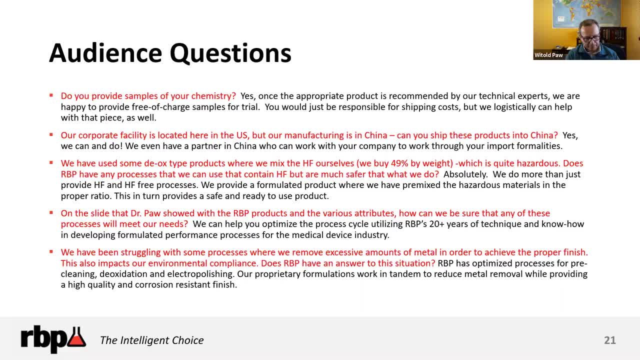 cases, remedies to those situations. Okay, All right, So we have not received any additional questions, So just a reminder to everyone listening that you can ask a question. Now's your chance to ask anything that you ever wanted to know about medical device chemistry but were afraid to ask. There was two more of our. 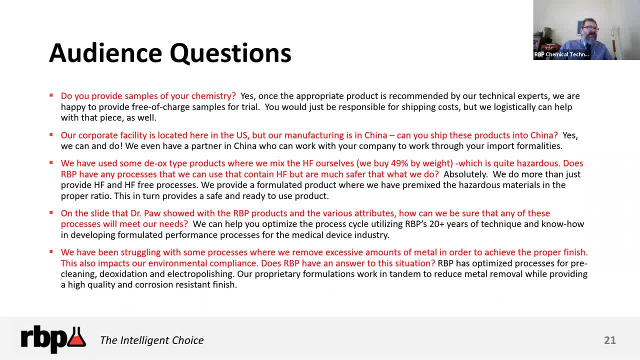 sample questions: The slide that Dr Pa showed with the RVP products and the various attributes. How can we be sure that any of these processes will meet our needs? Hey, I'm tempted to answer. You can never be. you can never be sure, but you can try And we have a. 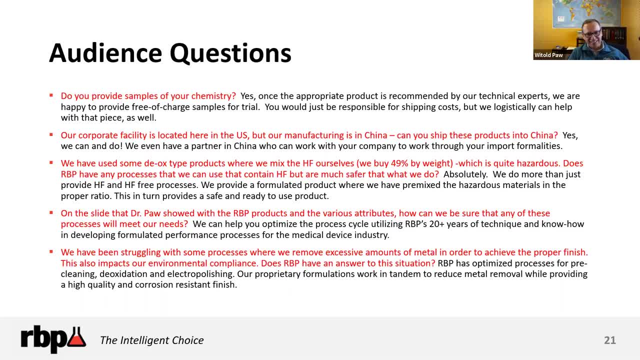 range of them, And we have. we have several, because at some point, what we had didn't work, So we came up with another one. So, and again, if one of the products cannot do the job for you, then there is another one to be formulated, and and that's what we'll do. 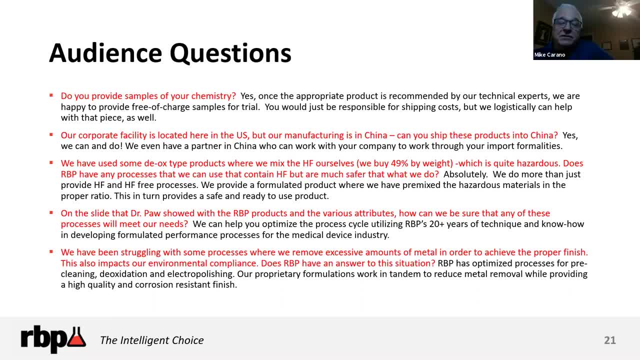 Okay, Yeah, If I might add to to that point about how we optimize the process cycles, like you know, we could get uh, two, uh samples of Stencin from two different companies And they'll say we'd like. 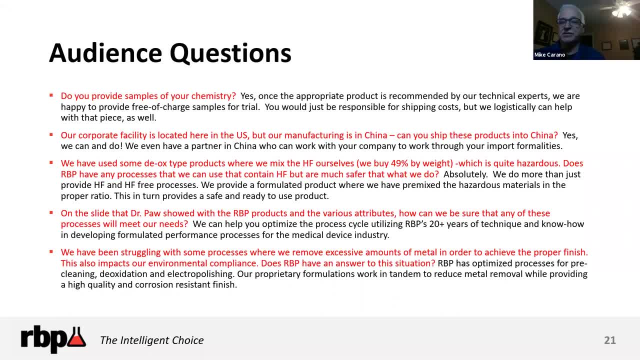 to have the electro polished and we could say: here's our. we take one of them down one of our lines and it will come out perfect. we take the other step and it doesn't come out perfect. why doesn't it both nitinol? maybe the nitinol came from the same metal producer, so why is it different? it's. 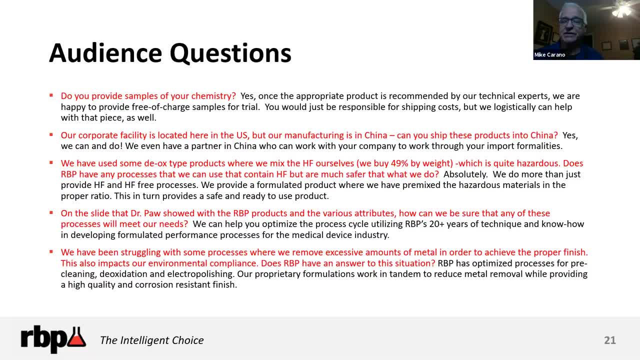 different because of how those parts were either cut or heat treated or whatever it was done differently, you know, within that particular process. so that's where we come in. those are the variables are are that can impact the performance of any processes, which is why we, you know we can provide you with this help. we've been doing this for 20 plus years and Vito can. 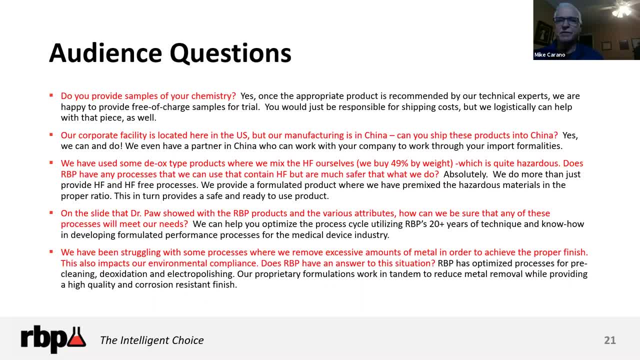 comment after. but how many samples and customers that we've worked with just in the last six months doing this very same thing. it's it's in almost triple figures. so we understand this. we've got a good understanding of technique and know how how chemistry works, how the inhibitors and 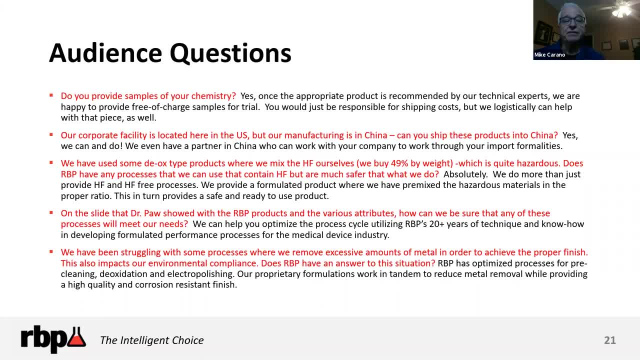 functional, you and materials work. but I also want to stress one other thing. when people say, well, I want to, uh, they send us a part or they call us and they say I want to electro polish, well, you know, there's, there's, it's a process, there's more than just to the polishing spot. there's the cleaning, there's. 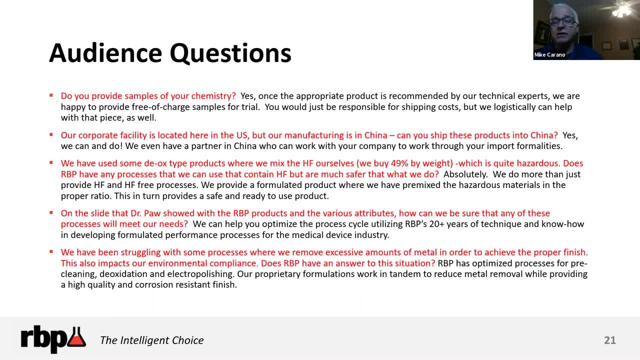 the deoxidation. so what I'm saying to you is: you know, when you just say electro polish, there's more to it than just that. you know, I like to fly a jet airplane too, but I'm not going to be able to fly one today. I'm going to have to prepare for it, I'm going to have to figure out. 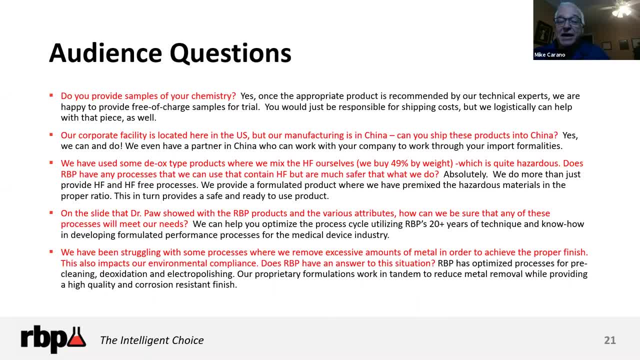 get the proper training before I can do that. so we we want to make sure you understand up front. it's, it's a process, and we again develop the, if you will, pre-cleaners and the deoxidizers that will help you gain a successful performing medical device that meets the, the F you know. 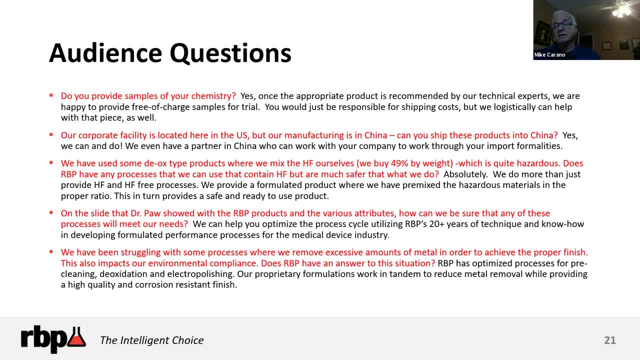 the F-21 29 corrosion resistance specifications. all right, okay, uh, we're just going to go ahead and go through this last question here, uh. before we do, though, a reminder to everyone that you can always find out more information about RBP chemical on our website, rbpchemicalcom also. 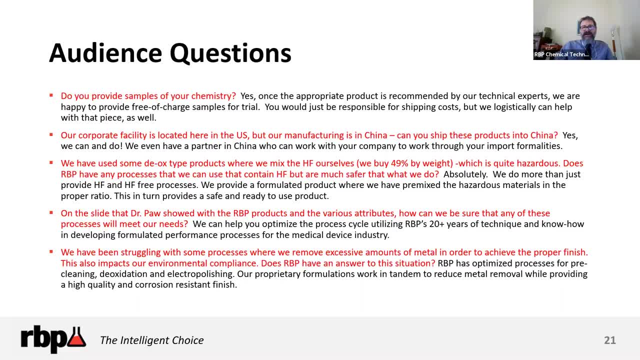 a nice way to contact us, as well as through the website, again, that is, rbpchemicalcom. uh, so the last question we have on here. we have been struggling with some processes where we remove excessive amounts of metal in order to achieve the proper finish. this also impacts our 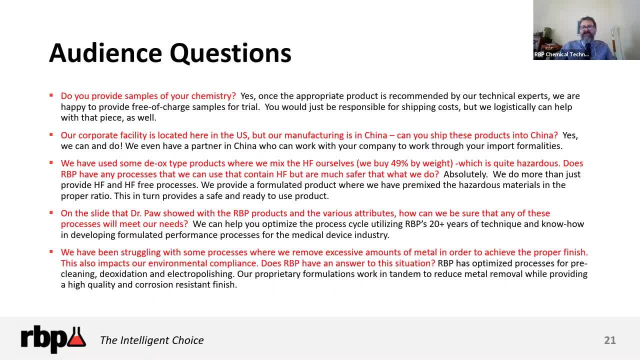 chemical compliance. does RBP have an answer for this situation? we do, and if we don't, we will look for it. uh, you know this is, this is a difficult situations because, uh, I'm not going to claim that our products will work for all parts, because parts uh are so different, you know different.